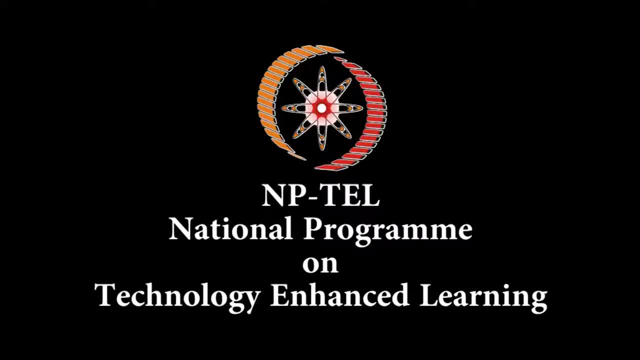 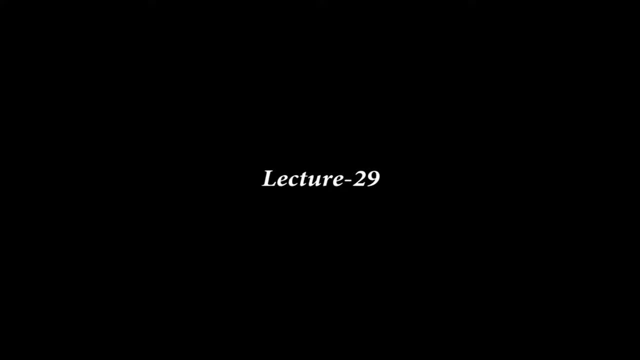 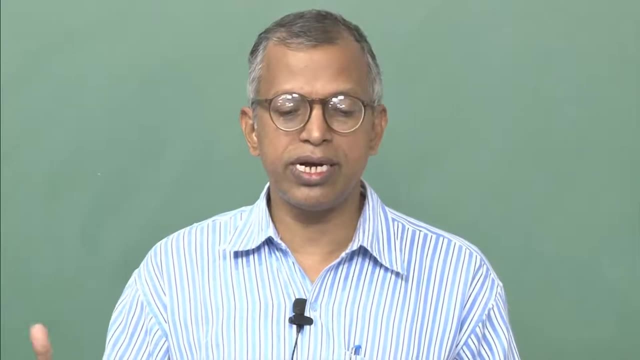 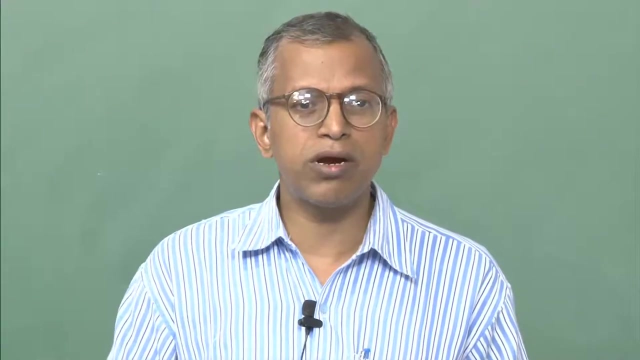 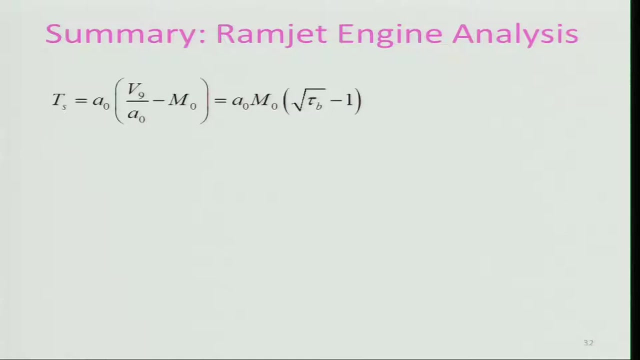 Let us summarize what we have learnt in the ramjet engine analysis. We have basically derived an equation for various parameters like specific thrust, thrust specific fuel conjunctions and other efficiencies. If you look at this thrust specific fuel conjunction, we have looked at it and derived this expression. You can note from this expression that thrust specific 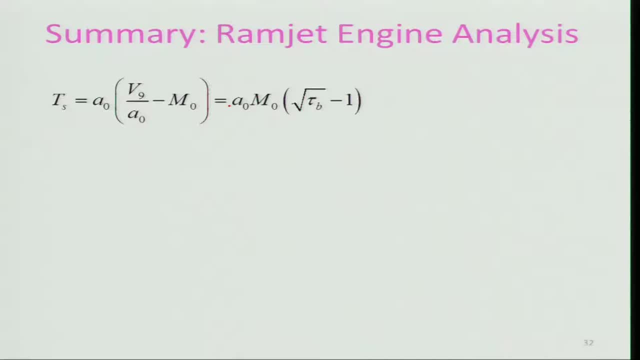 fuel conjunction is dependent on the altitude. If you look at A naught, and it is the altitude which will tell us whether it is what temperature and flight mach number. and it will be dependent how much heat you have added the tau p, that is, the burner, or what is called combustor. 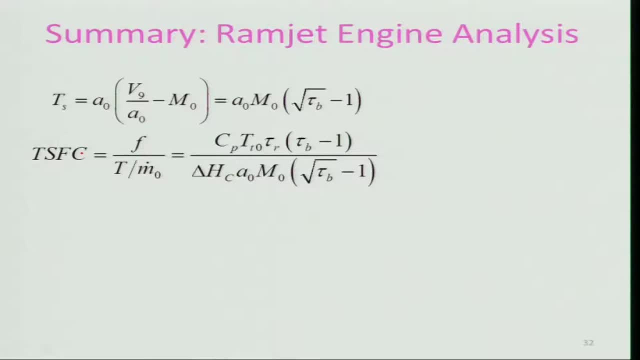 So similarly we can find out expression for TSFC. and these are parameters. Apart from this, what you call tau b m naught A naught. it is also dependent on tau r, but it is again function of flight mach number And, of course, the kind of fuel you are using, that is, heat. 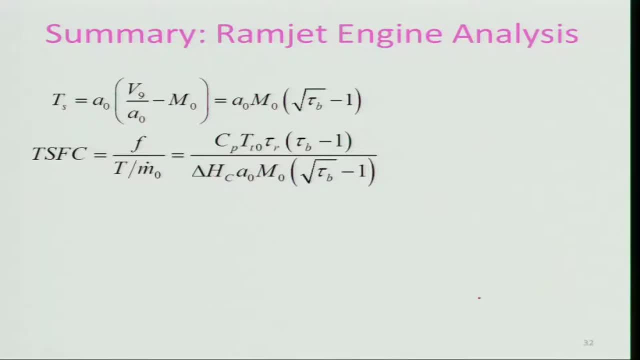 of what is called combustion And we have looked at propulsive efficiency and of course here we have using another parameter that is tau lambda and apart from tau r, So thermal efficiency it is really does not depend on the tau p When I am saying tau lambda, tau b is, you know, inside this propulsive efficiency. So 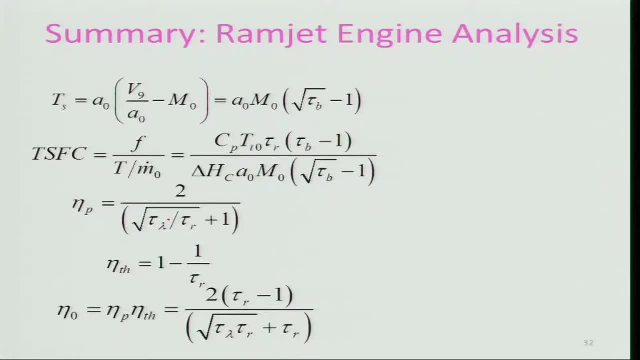 and overall efficiency. nothing but you know. multiplication of propulsive efficiency, thermal. What we will do with these equations? You can say: look, we have derived it. but our objective is to carry out a parametric analysis So that we can see which parameter is important. 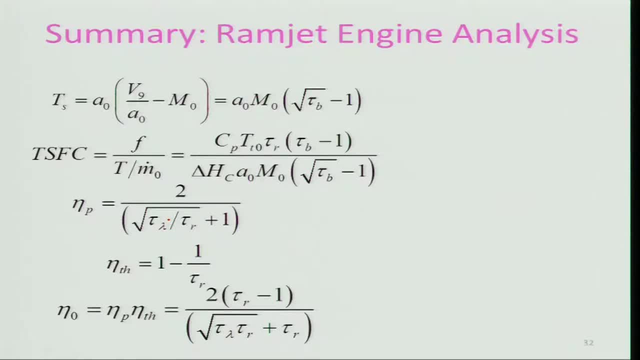 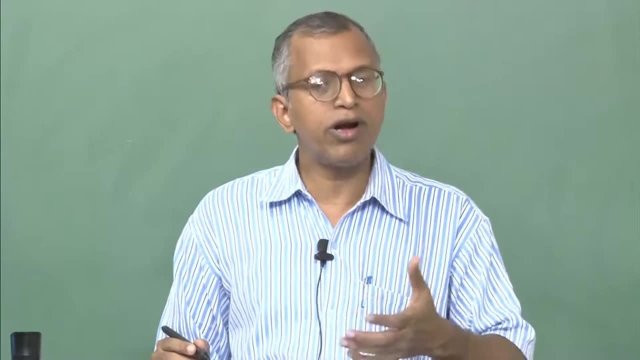 how to optimize and how to go about under ideal conditions, And that is why this is known as on design analysis. This can be used as a tool for design analysis, And keep in mind that we do not have any geometry, we are just talking about. 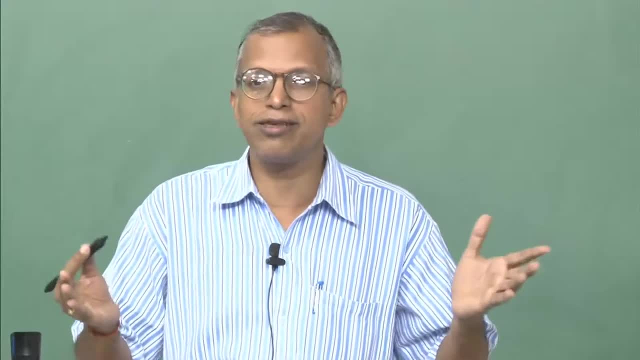 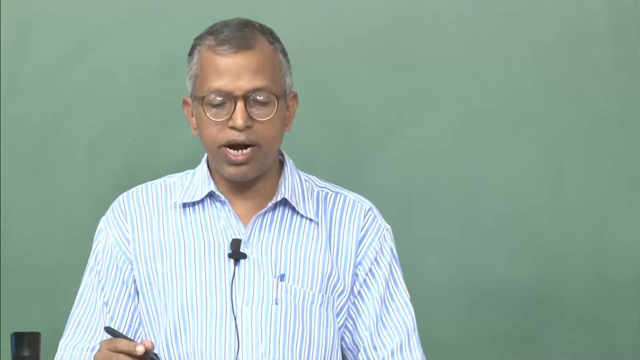 therefore, this sometimes known as rubber engine, you know, like nothing is there, but you are thinking it will be there and then looking at it. So what we will do? We will look at parameters and we will take this, you know, data, that is. 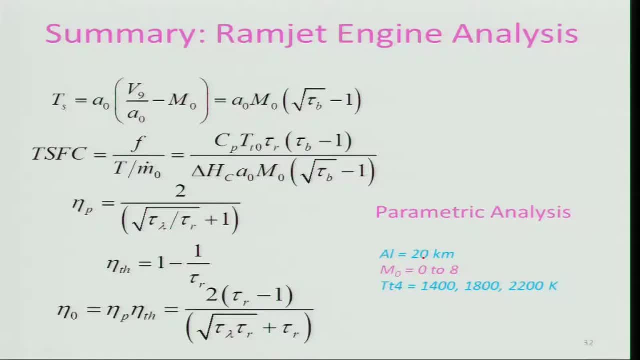 altitude. Let us say a ram jet is flying at altitude 20 kilometer. generally it will be till higher altitude and Mach number we are varying 0 to 8. of course 0 I cannot say because I have just taken, you know, just to completeness say right. 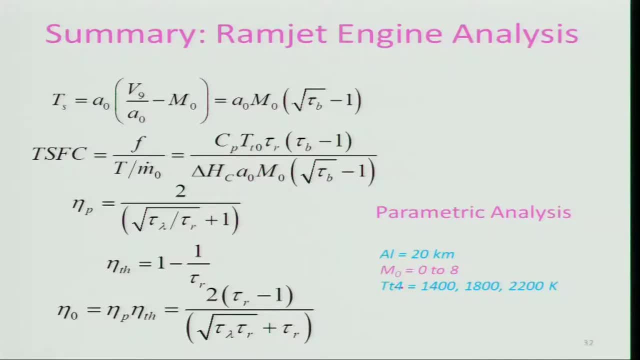 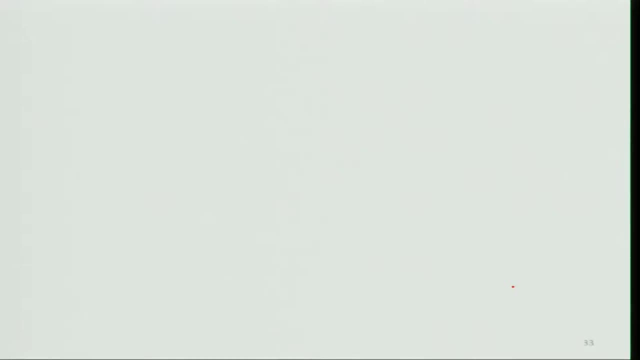 And T, T, 4, that is the turbine. sorry, that is the exit temperature of the combustors: it is 3. we have taken 4.. 1400, 1800, 2200 Kelvin and we are basically, let us vary this use. this equation may be. 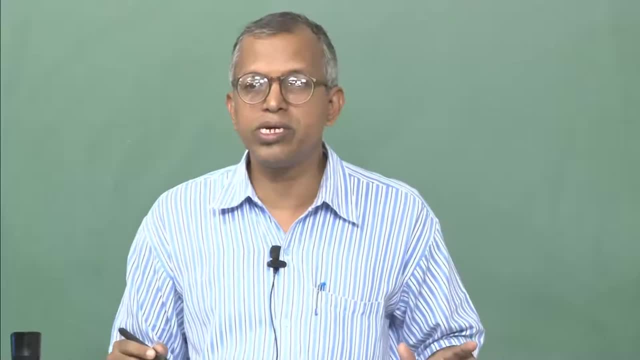 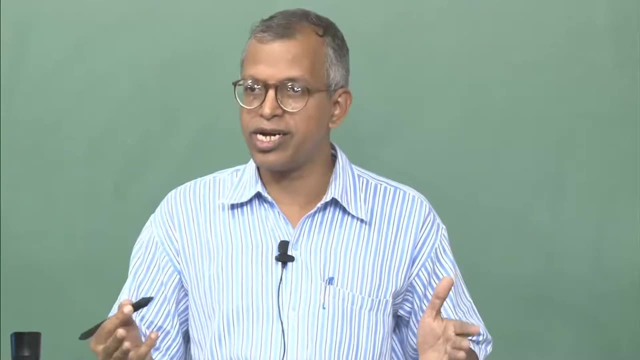 in a computer program or something to do. a lot of calculation one can do in hand, But generally you can write a small program and then generate data and plot it and see how it is varying and analyze those data. also. Plotting is not enough, but you will have. 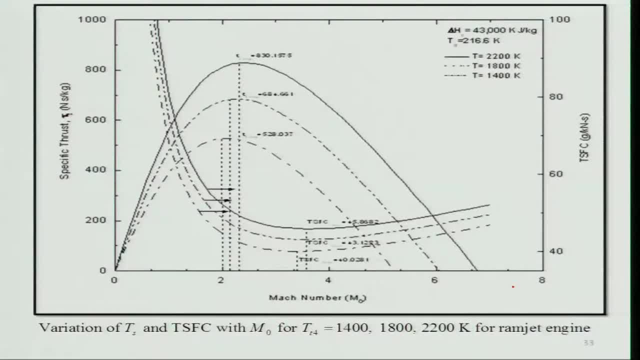 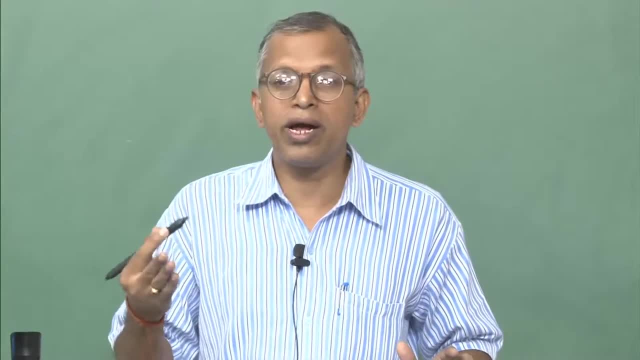 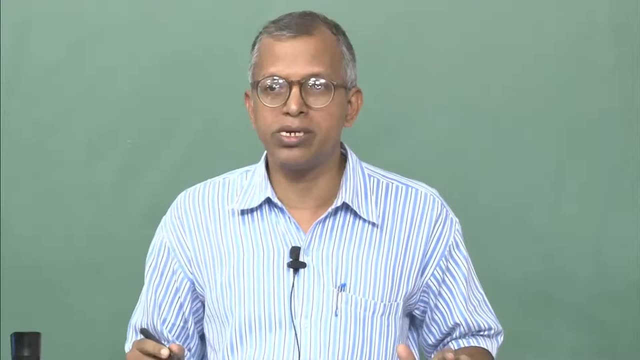 to derive some inference from the data. As I always said, that all information you know cannot be converted into knowledge, of course. rather, information does not mean knowledge. knowledge has to be obtained from the information. all information are not data right, So you need to understand that. So let us see that. 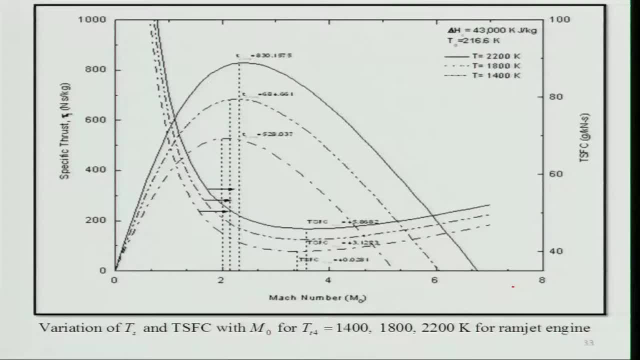 what we are doing here. we are basically plotting the specific thrust versus the Mach number. right, It is a similar value, only there is a little shift in the maximum specific thrust at a little higher Mach number. right, only that is the difference, but it is similar, right. 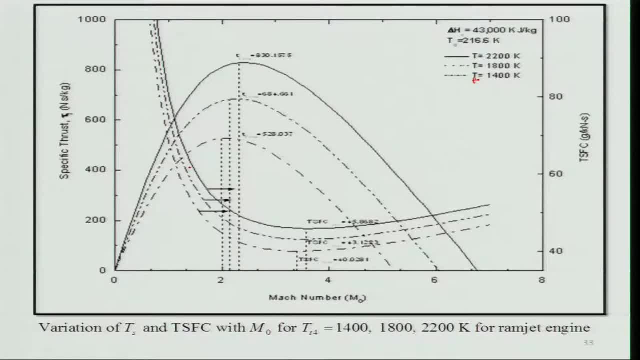 But if you look at why it is so? because as the Mach number increases, right, what happens? you get the ram pressure in case of ram. So the pressure is higher and you will get The higher thrust. right, of course you are adding it, but as soon as it will, or when? 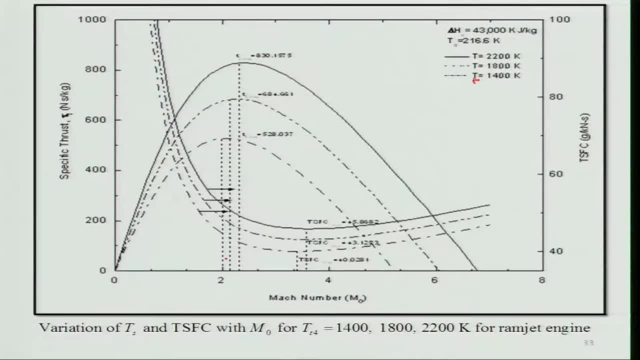 it attains a maximum value like that is optimum Mach number. basically, then what happens? why it decreases? because suppose you are flying at, you know, let us say 3 Mach number, right for a lower temperature. So what will happen at the temperature at the exit of your air? 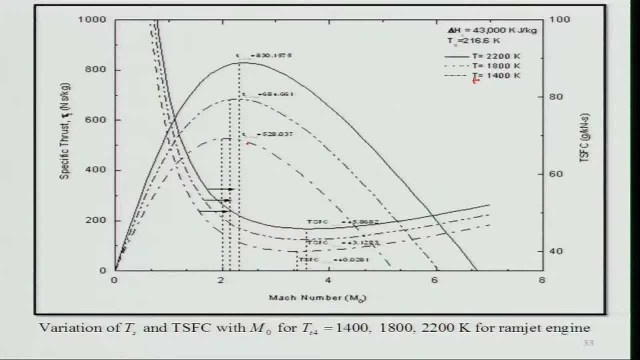 intake, it will be much higher And then there is not much heat. you can add to the well, because the restriction on the temperature 1400 current right and as it is. So then you know like what will happen. some of the things will be really decreasing, out right decreases and it became whatever your 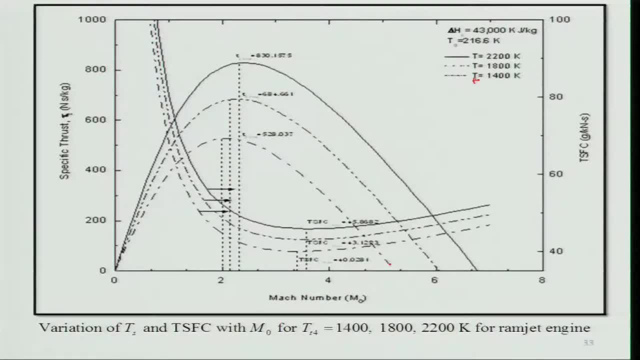 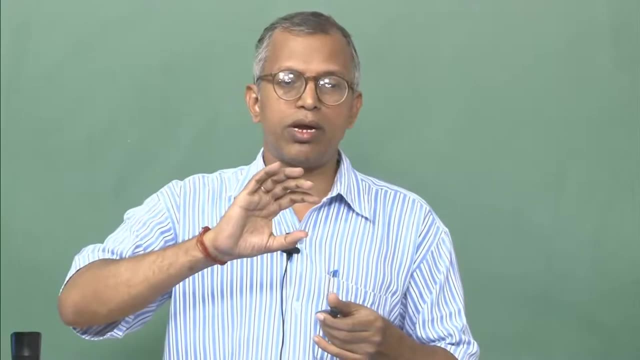 energy you are giving and at the higher Mach number whether it is coming. So it cannot be converted in to this drag. if you look at the inlet drag will be much higher In this case. what we are doing, we are saying this exit thrust because the what you call high velocity hot gas right? 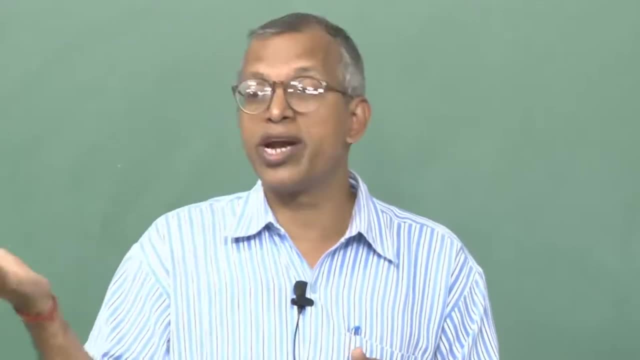 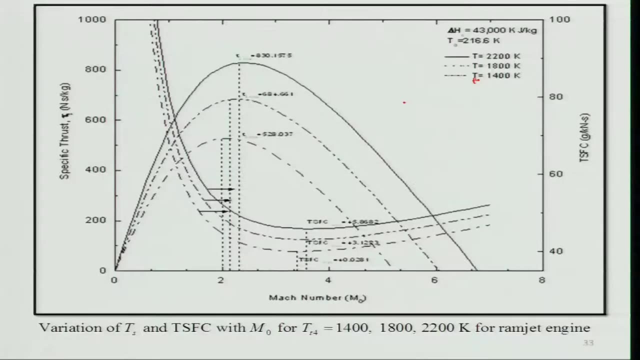 is coming out of the chain right And as a result, you are getting a thrust. but here, as I am increasing, for example, like if I, as I am increasing the flight Mach number, then your thrust will be decreasing right. For example, if you look at m 9 v, 9 minus. 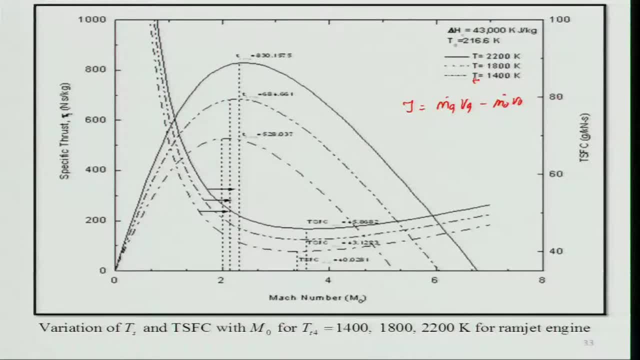 m naught v naught. So, as I am increasing this Mach number, you know, if I am increasing Mach number, what happened? this became high as compared to this, because this is limited by a- how much heat you can add and how much you know, kind of things. So therefore, as 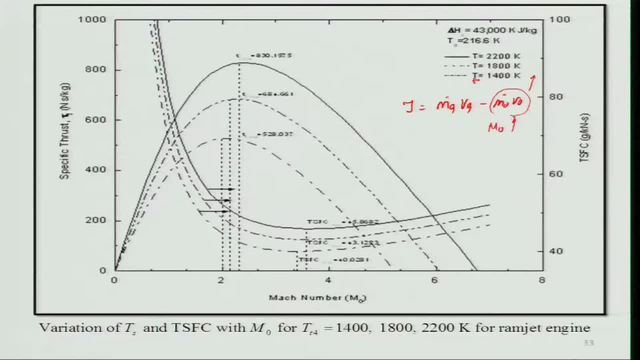 a particular heat input, you know this will be goes on increasing. So therefore, as a particular heat input, you know this will be goes on increasing. So therefore that will be negative heat. therefore this is decreasing right that make sense to you, any doubt? because this part is decreases, because your inlet drag. 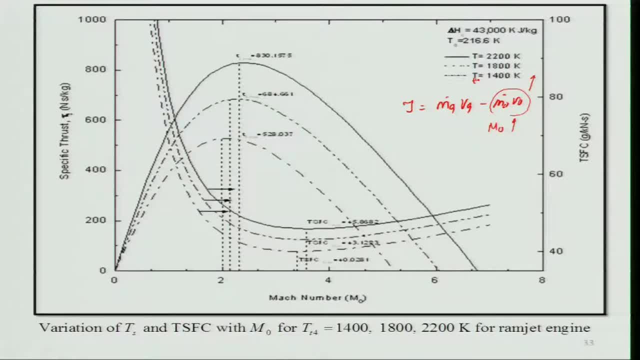 is higher with the higher Mach number for the same engine. keep in mind same engine. So there is another interesting thing. you can look at it. that is what we call the specific thrust. it decreases, right Like at a lower Mach number. it is quiteau. 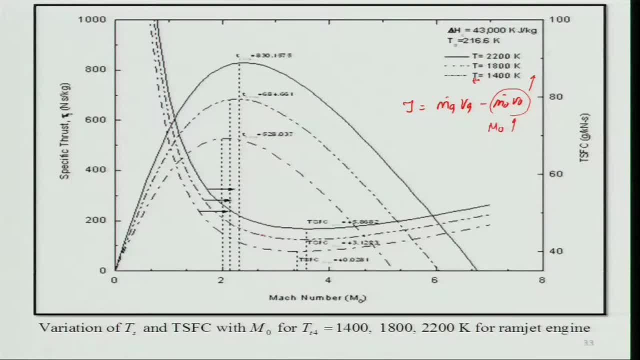 There is a another thing, interesting thing. you can look at it. that is what you call the. it is quite high and as it Mach number increases- right Mach number I mean- then it reaches a small value, then after that it goes on increasing, but in a very, very low. 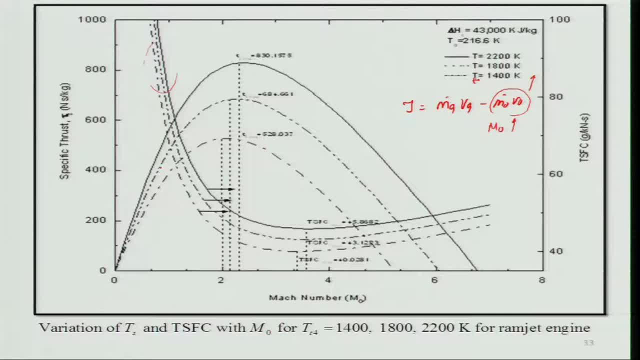 So, if you look at, but in this region, like where the Mach number is very low, although you are getting a specific thrust in this Mach number, but the TSFC is very, very high, but when what happens at the 0, 0, it will be infinite, very, very high. that means it is. 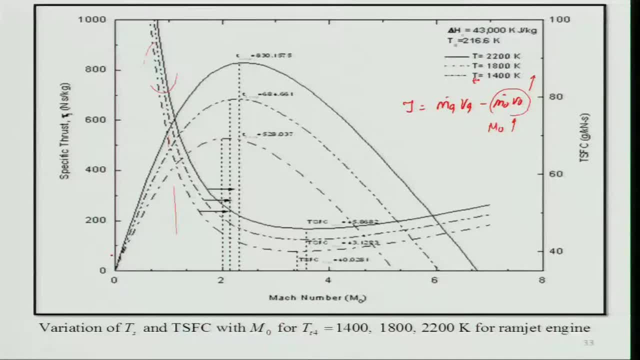 having no meaning. you know like that way. Therefore, you know the problem of 0 static thrust, as the Mach number 0 is a really a critical problem for that I am guessing. So you can also note that TSFC goes on decreasing, as basically you are decreasing the temperature. 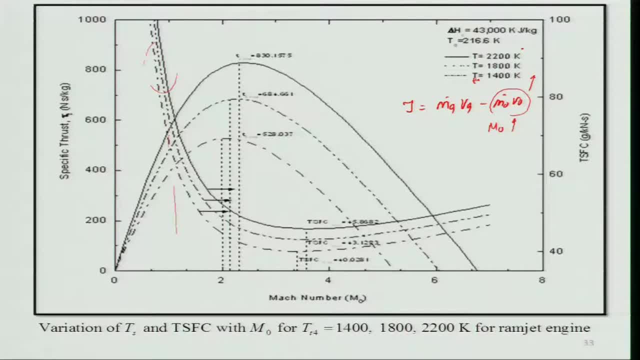 rather than, in other words, when I am increasing the exit rate, Temperature from the combustors, the TSFC goes on, which is obvious because as you want higher temperature, you need to can do more fuel right. So if you look at the propulsive, 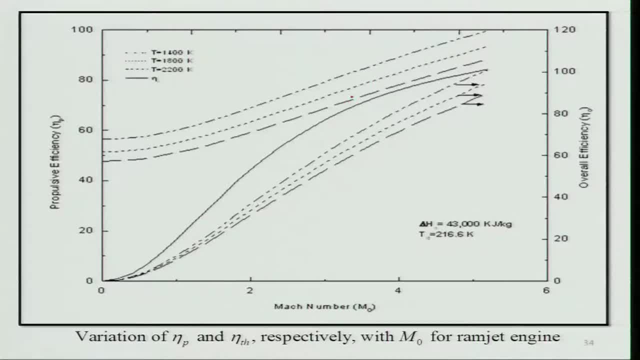 efficiencies. these are basically what you call is increases with the flight Mach number for the same temperature. However, the thermal efficiency does not depend on the Mach number, on the increase in temperature, but it does not depend on the thermal efficiency. But it does depend on the Mach number because it goes on increasing with the flight Mach. 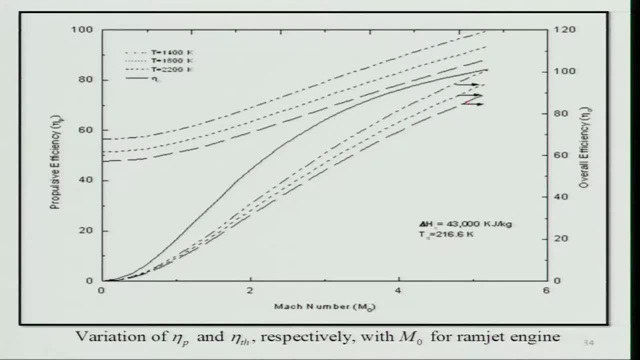 number and overall efficiency. multiplication of 2, you can see these are the overall efficiency, which is increases with the flight Mach number, right? So I mean, this is the thing what we have learnt in this, and we can also carry out several parametric variations. try to understand. 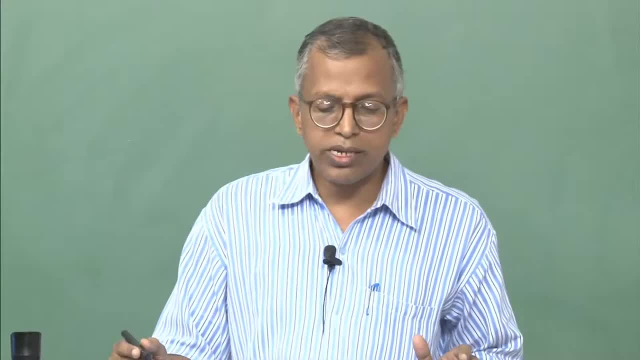 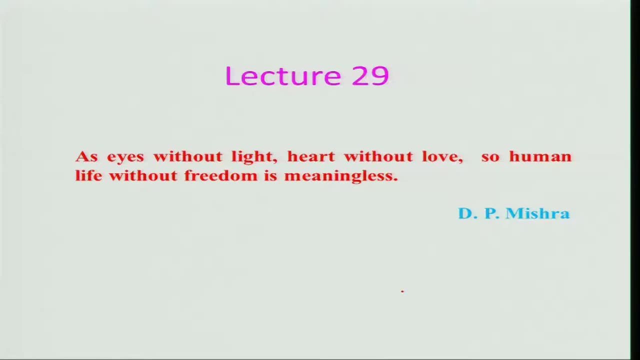 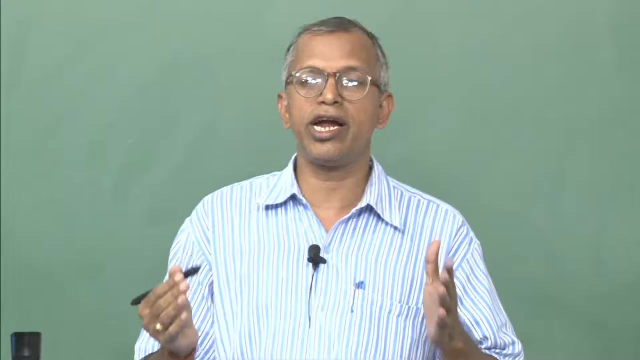 what is happening with this equation. So let us start this lecture with a thought process, as eyes without light, heart without love, So human life without freedom is meaningless. So let us look at what we learnt in the last lecture. we have basically looked at ramjet engine and carry out the analysis and we have 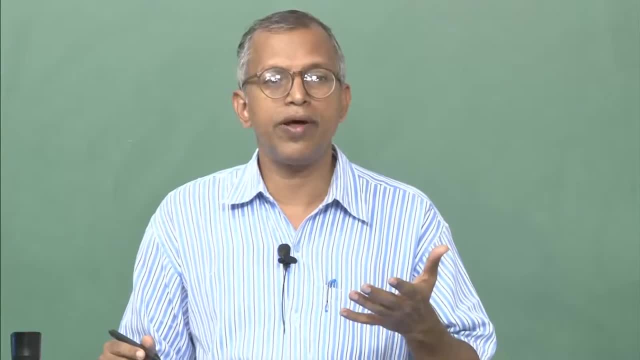 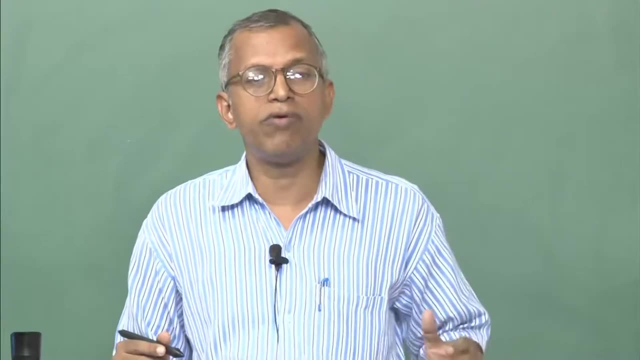 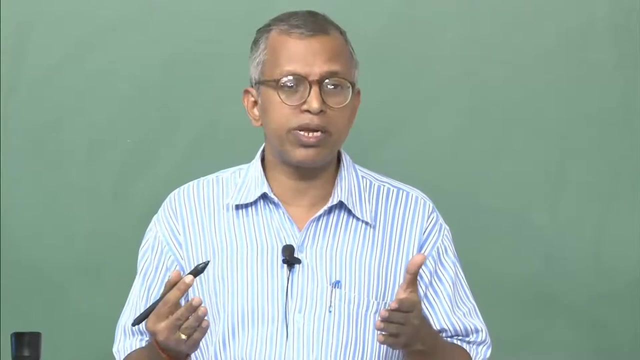 also looked at a parametric studies right and how this thrust or the specific thrust will be varying with Mach number. So we have looked at a range of temperature. temperature means combustion exit temperature, combustor exit temperature and we have looked at propulsive efficiency, overall efficiency. 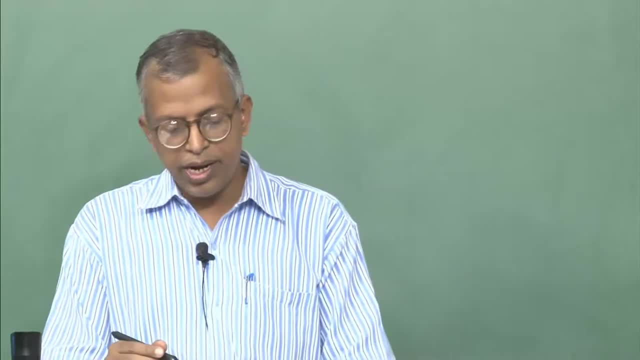 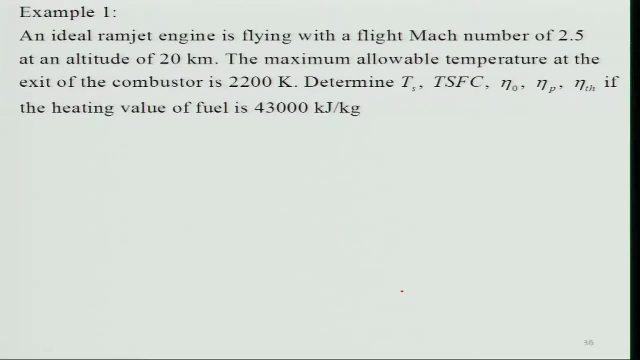 and thermal efficiency. Now what we will do, we will be looking at basically an example and use those expression and do that. and I will take the same example and use a another method. you can say: this is the method 1, I am doing that now, method 1.. 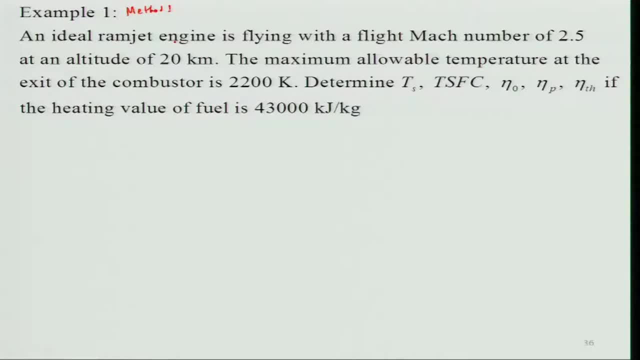 So what is that? an ideal ramjet engine flying with a flight Mach number 2.5, altitude of 20 kilometer, maximum allowable temperature is 2200 Kelvin and we will have to determine specific thrust, thrust, specific fuel consumption and all other efficiencies. right And these. 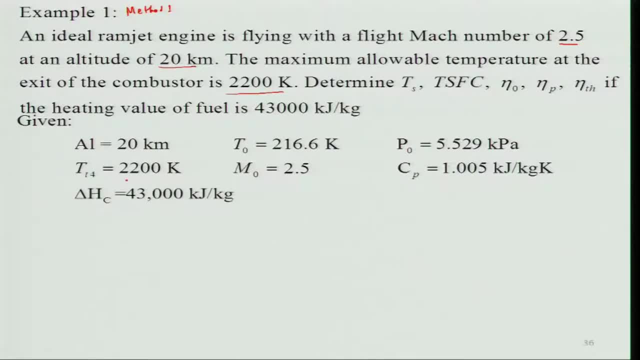 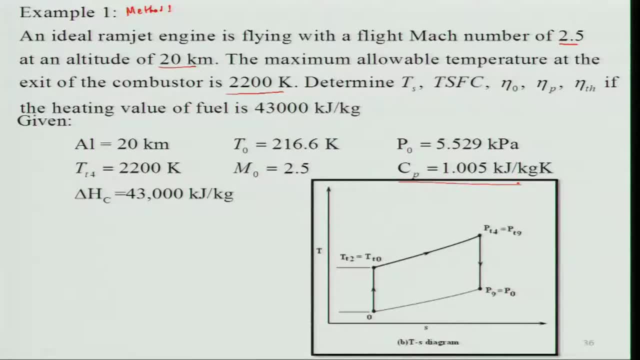 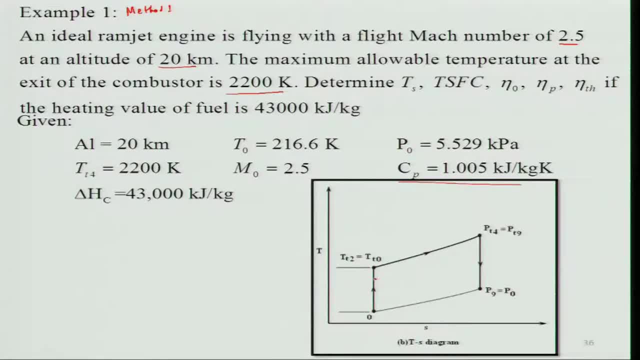 at s diagram. you know, like 0 to 1 is your basically compression or ram compression, And this is the heat addition combustion from heat station 2 to the 4 and this is your expansion is north right. So what we will do, we will basically know. 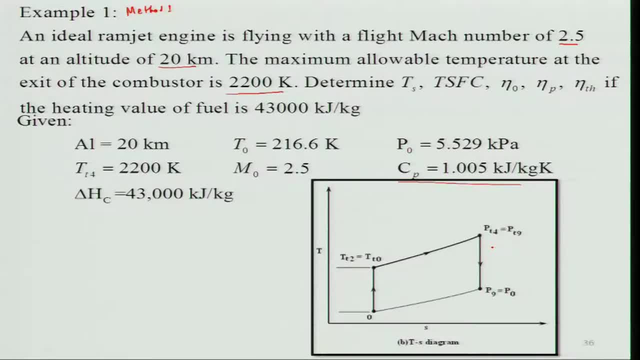 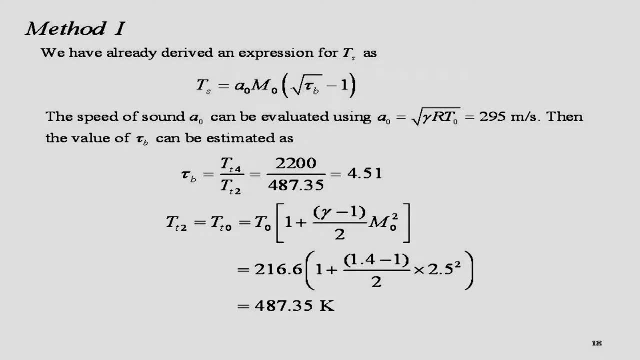 these values. we will look at it kind of things and then do the next project. So what we? method 1: as I told you, we have already derived those expression for the specific thrust. So what we will do, We will just, we know these values. this is 2.5, do you know that? 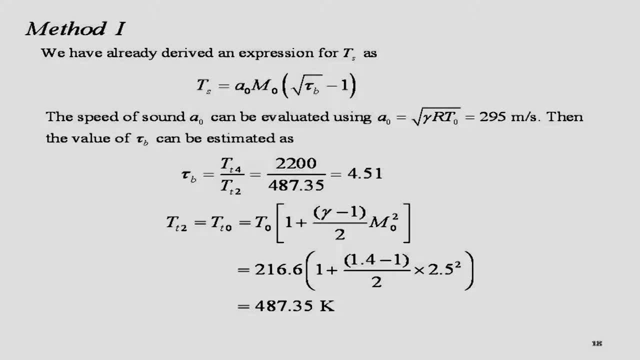 and we will find out A naught. of course. we know altitude, we know the temperature and knowing that we can find out A naught is equal to root over gamma r t. So that is, A naught is equal to root over gamma r t naught and we get this 2.5.. So we know that and if you 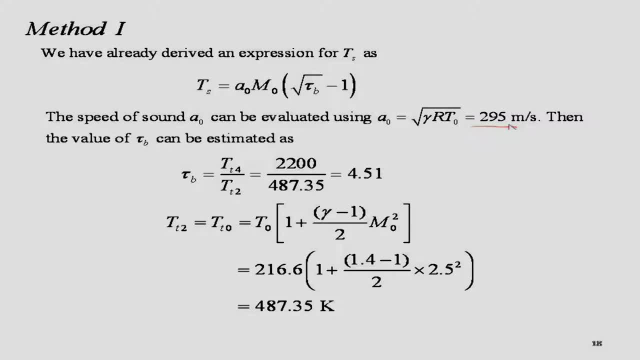 look at this specific thrust is. I mean, like you know, then we need to find out tau b. tau b is what is that? by definition, it is t t 4 by t t 2. So that is 2200 Kelvin which is given and we need to find out t t. So how we will find. 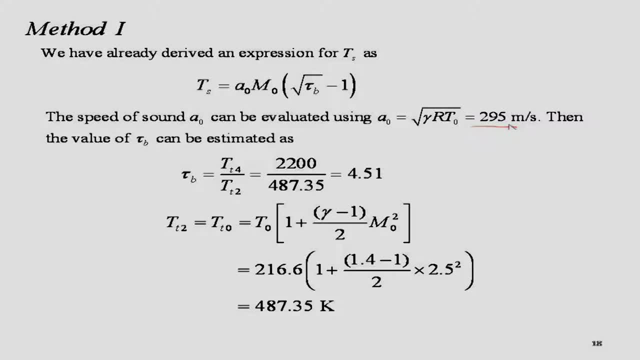 out t t 2?. t t 2 is equal to t t naught. we know t naught into 1 plus gamma minus 1. divide by 2 m naught square. we will substitute these values. this is given from the altitude 216.6. 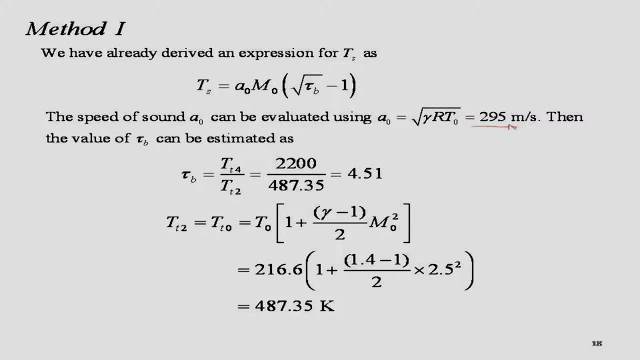 Kelvin. when you substitute values, we will get 487.37 Kelvin And then you substitute, we get these values and once we get these values, we know basically, whatever the parameter in specific thrust, that is, A naught is known, m naught is known. 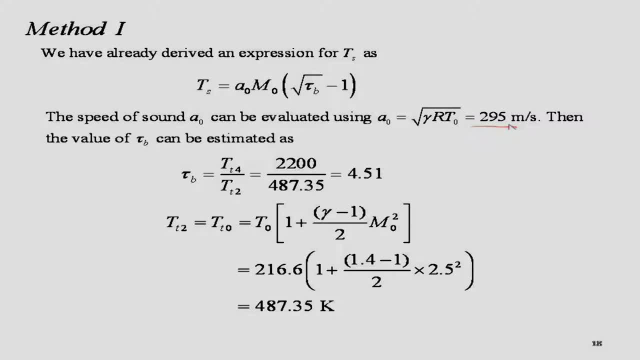 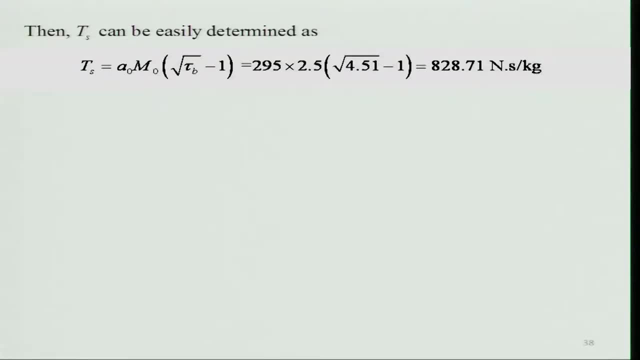 tau b is known, So you can substitute those values and get the specific thrust. So if you look at, I am just substituting these values and then I am getting 8 to 8.5.. It is 8.71 Newton per second per kg because 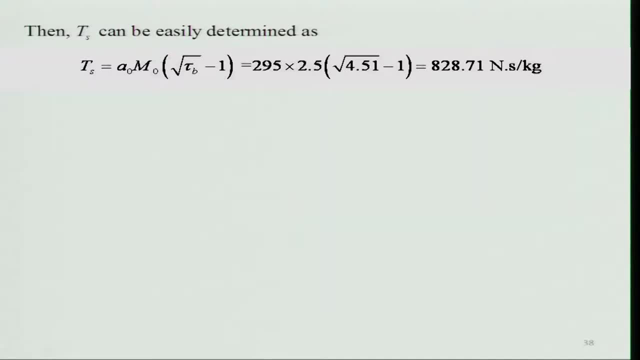 it is per unit mass of air flow rate. its specific thrust is being thrust divided by the mass flow rate of air which is entering into the inlet of the engine. So the expression for T, S, F, C can be used to evaluate its values. we know this by definition: C, p, t, naught and. 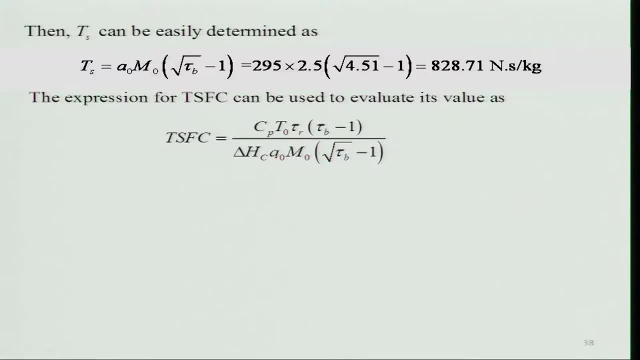 tau b. Now let you evaluate it. delta S is known, A naught is known, m naught is known. you just substitute these values and you get. So do you know this tau r? tau r is a very 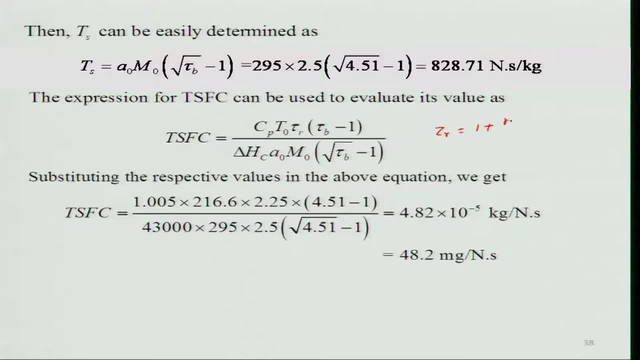 simple thing, what you will have to do. tau r is equal to 1 plus gamma minus 1 divided by 2 m naught square. So I know these values, I know gamma, so I can find out very easily. 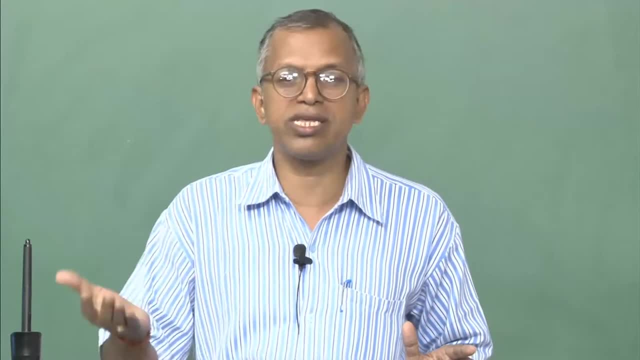 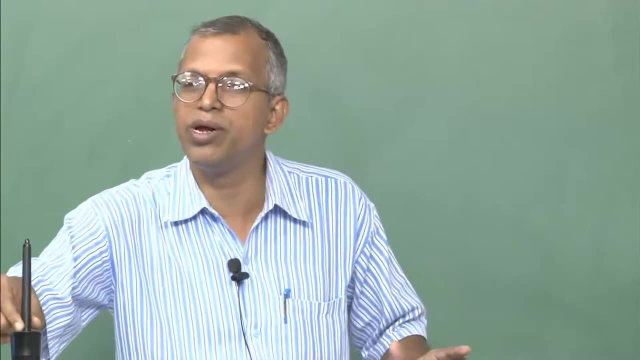 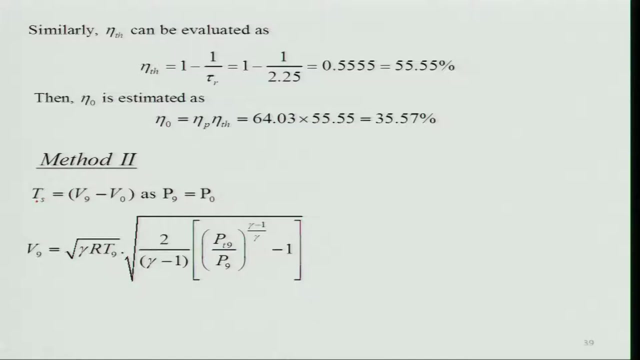 I can find out very easily. then you can adopt the method 1 and which is essentially designed for a what you call parametric studies, and in nowadays computer is available. you can use that very easily without really thinking much. So what we will do, we will basically looking at specific thrust- is equal to v 9 by minus. 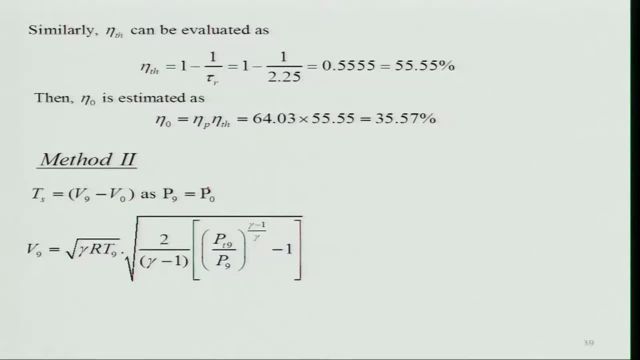 v naught and of course we are assuming v 9,. what is this v 9,? v 9 is root over gamma r t 2 divided by gamma r t. So that means I need to determine this t 9,. I need to determine this p 9,. do I know? 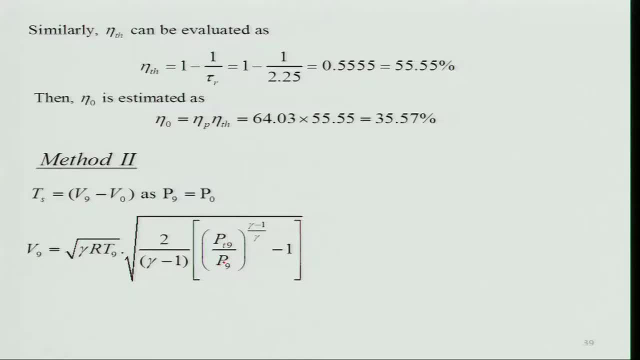 really p 9, p 9. I know it is nothing but your p naught. but do you know the p naught? you know the r t 2, so you know the p naught. So similarly, we will have to find out p t. 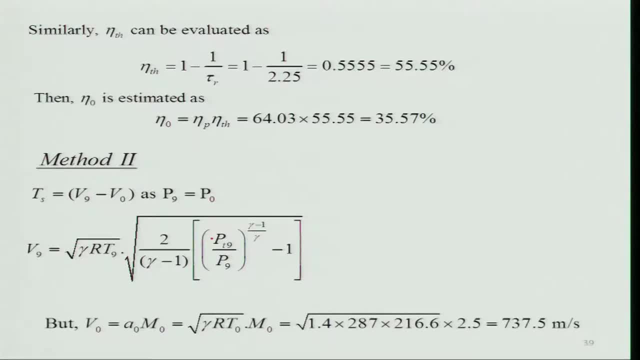 9. And v naught we need to find out that is a very simple one, which is same as that of the previous method. that is, a naught m naught, and you just substitute these values, you will get 73.5, 737.5 meter per second. At least you are having a feel what is v naught? but 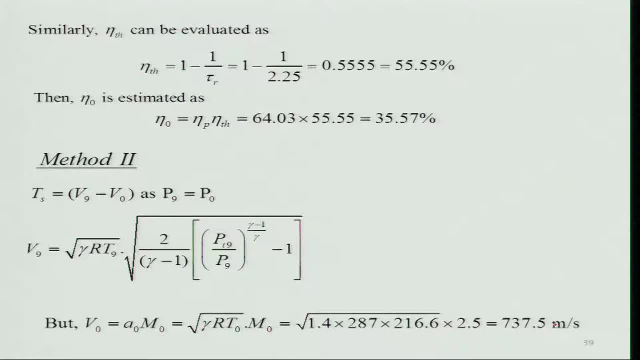 in that other method, you do not know really, you substitute the values of m naught and you do not know what is the, what will be the velocity with v naught. So that gives a feel and, as I told you earlier, what we will have to do. we will have to, basically. 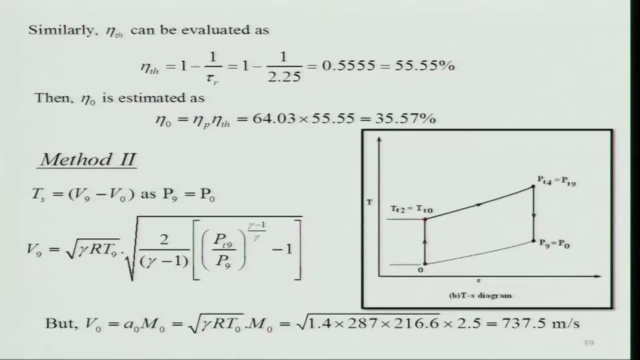 find out from here and go to this point, find out various properties, pressure, temperature, whatever it is required. Similarly, I will have to go this point to t 4 and then find out what will be the temperature T 4 if it is not given, if it is generally it is given or sometimes you need to find. 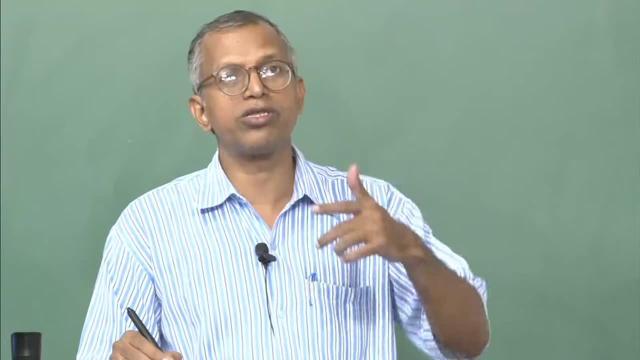 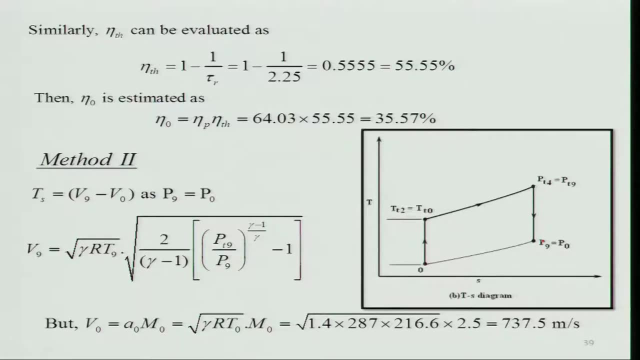 out. you know that you do not know really, and you will have to cross check whether it is that. And then, of course, this you need to know or you will have to find out. in this example or ideal situation, p 9 is equal to p naught. So you know, but in when you go, 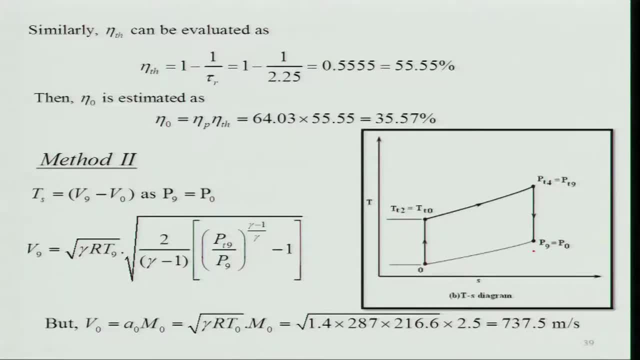 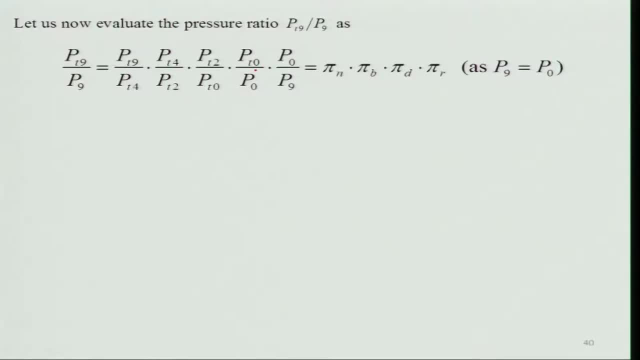 for real cycle. you would not be knowing this. you need to find out. p 9 would not be known some cases. So let us evaluate this p t 9 by p 9, you can use this method or you can go by some. 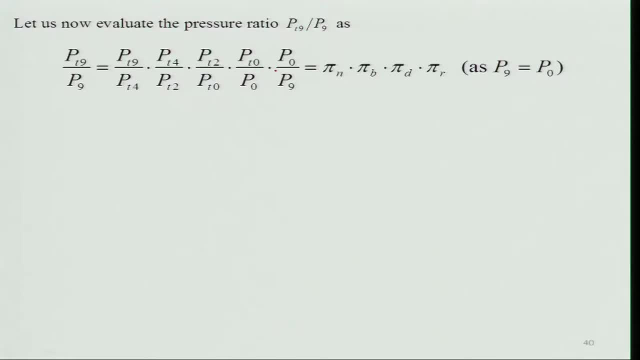 other method, also step by step. So these are the same thing I have done. So, if you look at this, pi d will be what? pi d will be 1, pi n will be 1, and what about pi b can? 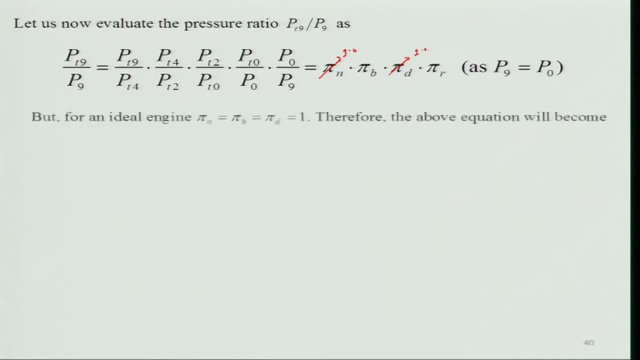 I say it is as a 1. Right, And pi b is also- will be 1 because there is no pressure loss in the total pressure loss in the burner. So this will be also 1.. So that turns out to be pi? r and pi? r you can. 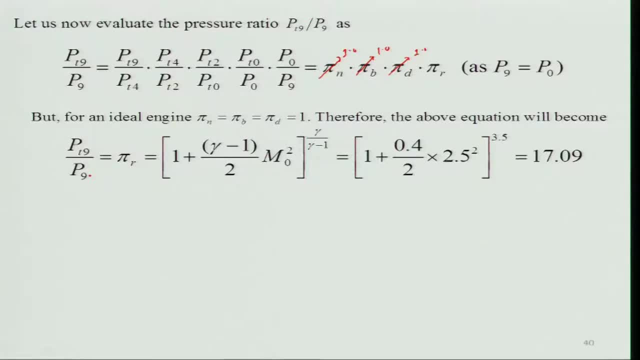 find out very easily, So that you know this pressure ratio and p t 9, you can find out. I mean, you need not to, you can really substitute these values and find out. m 9 is this much 2.5? and interestingly, this m 9 happens to be same as that of the what you called flight. 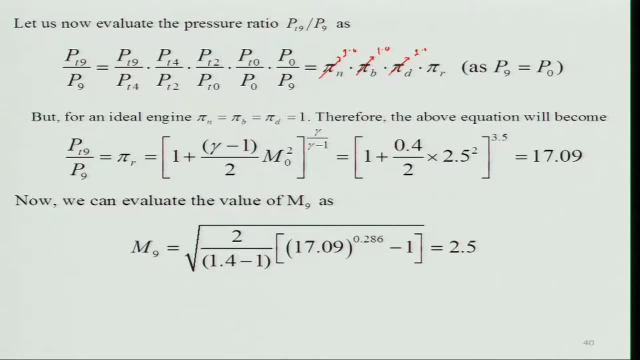 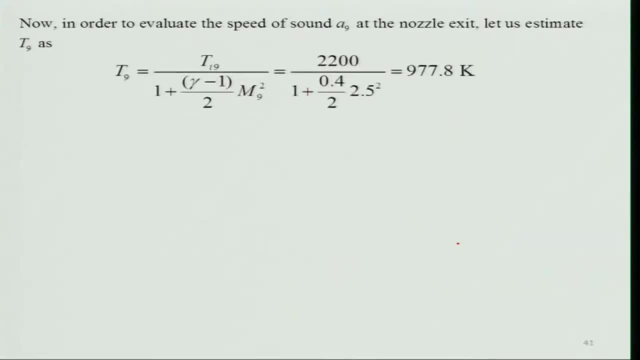 map and that you valid only for an ideal case. So now, in order to evaluate speed of you know sound a 9, I need to find out map T 9,. you can find out T 9 by this, what you call. 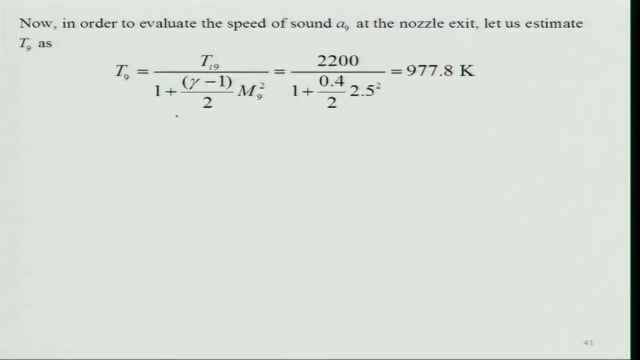 T 9 kind of things, and you will get that it happens to be 977.8 Kelvin. So if they have 2 equations above 2 equations, we can evaluate V 9. I know this V 9 and I know the m naught. 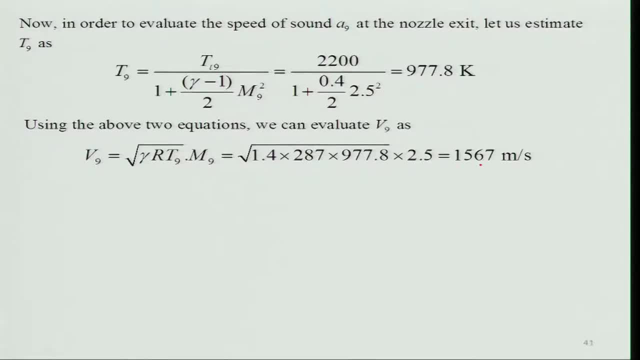 I can find out. So this V 9 happens to be 1567 meter per second and which is not same as the flight velocity, which is 700 odd numbers, right? So when you substitute these values, you know you will get 8 to 9.5 Newton second per kg and you will see that it is almost. 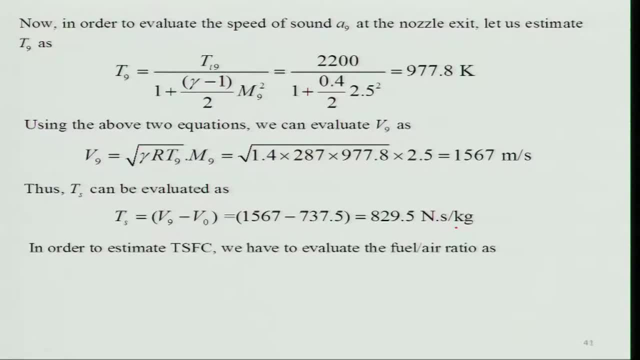 same as that of the earlier method. So in order to estimate PSFC, we can evaluate all those things: C, p, delta S c, T, t 4 minus T t 2. right, this is, we are not using tau b, tau r, but you can put that. 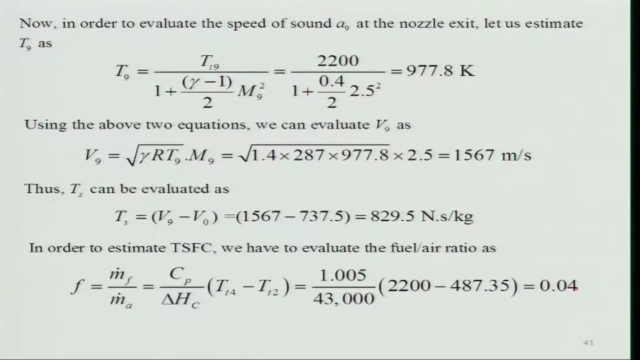 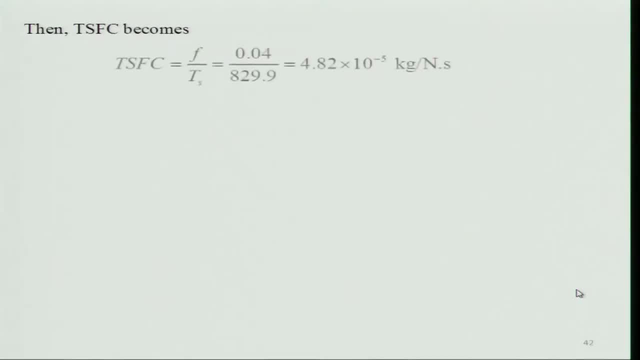 It is happens to be 0.0, 0.04, and keep in mind that this is what you call a ratio, right? So using this we can find out: PSFC is equal to F by T, s, that will be 4.82 into 10 to the. 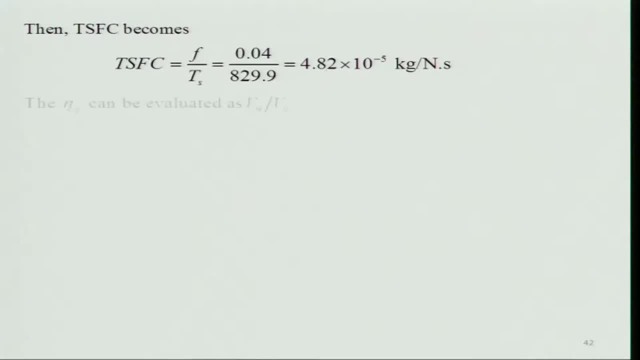 power minus 5 kg per Newton second and which is same as that. So propulsive efficiency can be evaluated as V 9 by V naught, right, So V 9, we know the V naught. So you can get the propulsive efficiency very And thermal. 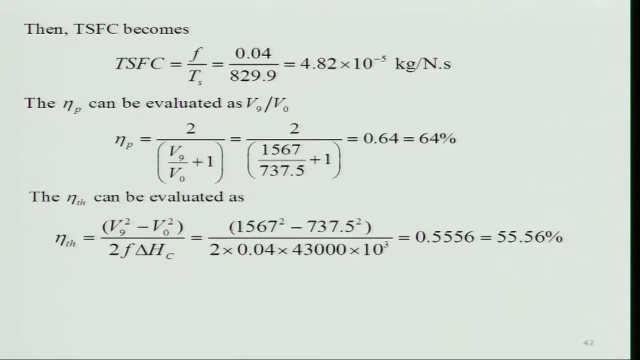 efficiency is same as that when you substitute V 9 and. but here you can see that what is the difference, you know, in that velocity and how much change in the kinetic energy is occurring. you can have a feel for it. where you cannot get there, it is just a number. and what will? 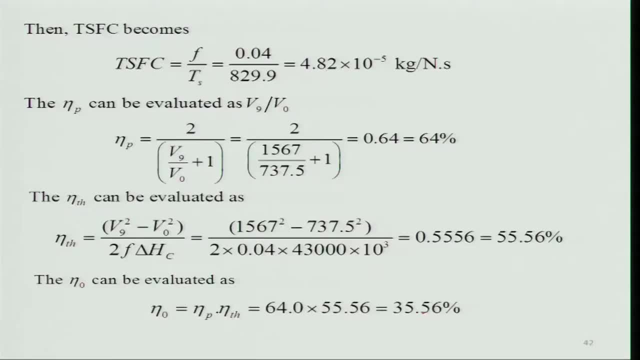 come. So the overall efficiency will be 35.6.. So what I am suggesting? that you, if want to have a feel, you will go for this method 2 and I would argue people to use in your exam and other places, the method 2, unless. 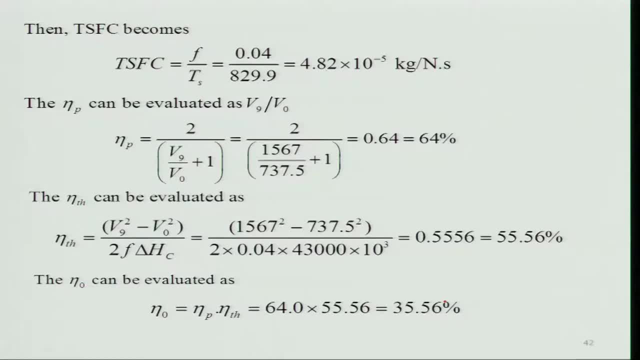 otherwise stated, particularly in some assignment. I will be giving in some questions where you need to carry out parametric scheme. Therefore, method 1 has to be adopted for those problems. Rest of the problems: the method 2 is that that is the last method of the three methods. 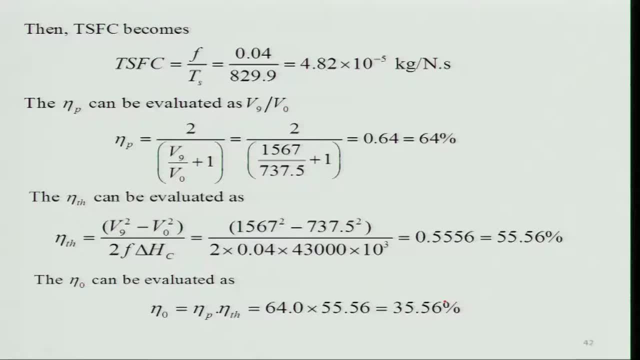 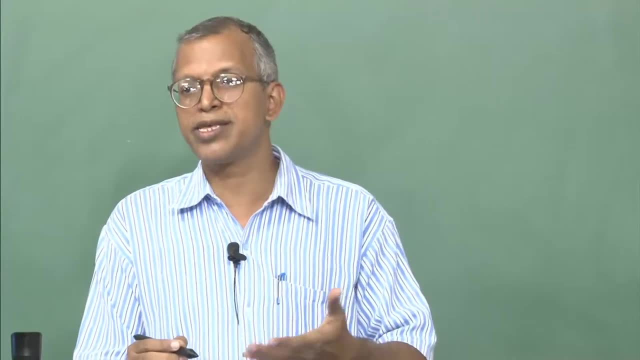 And I have given only little explanation about this method, but it is the most simple one. method 2 is to be adopted. is that clear to everybody? So method 2 gives a physical field. therefore, it is very essential you should do that to have a field for the what? 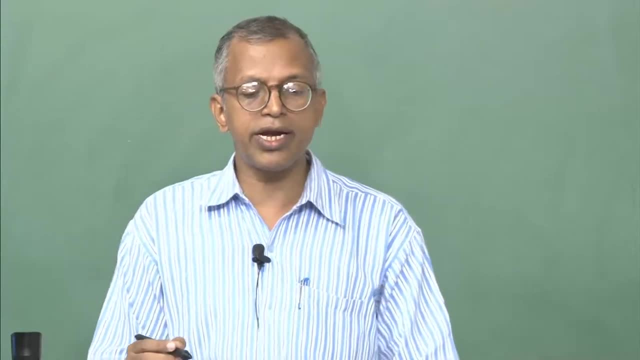 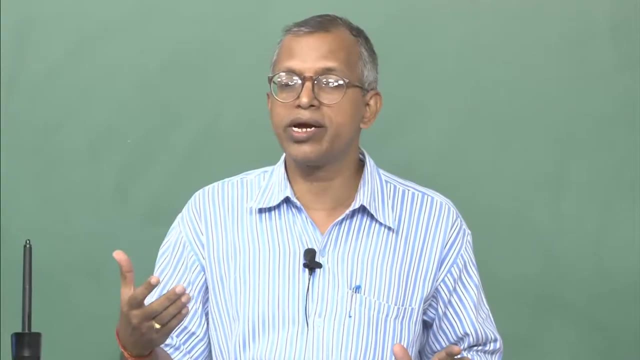 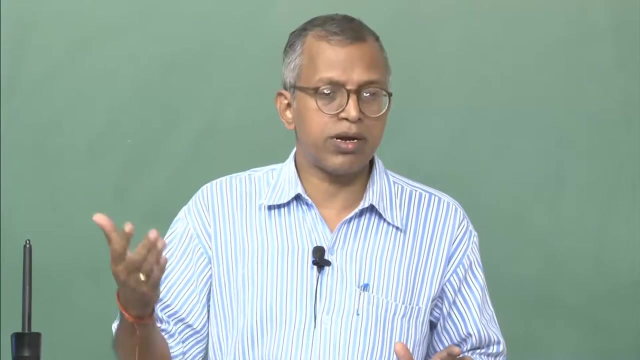 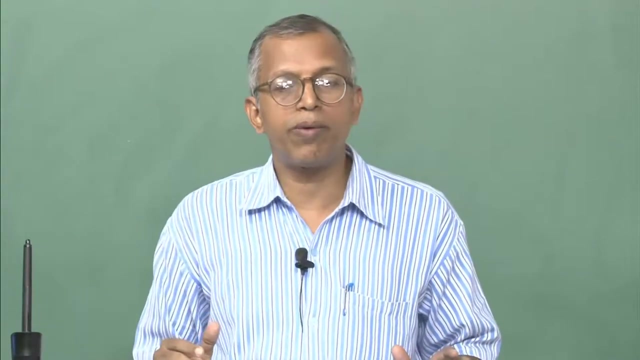 is happening what you want to exactly. So now we will get into the turbo jet engine. we know that in the ramjet engine there is always to problem to get the you know overcome, the problem of geospecific or the specific you know. So as a result, we cannot really make it a one from the what you call plane. 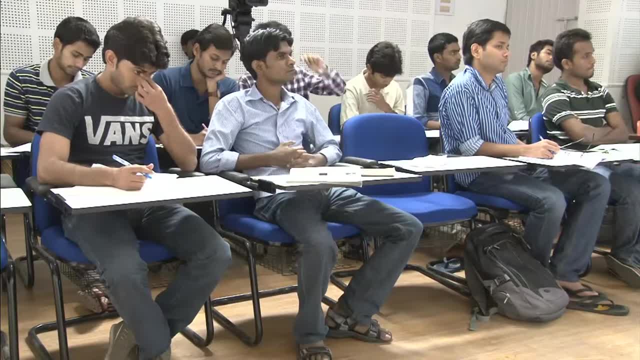 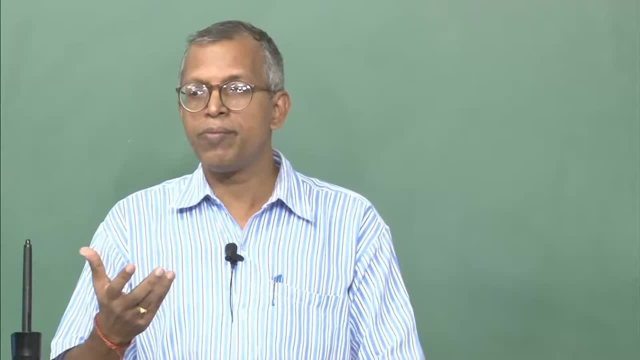 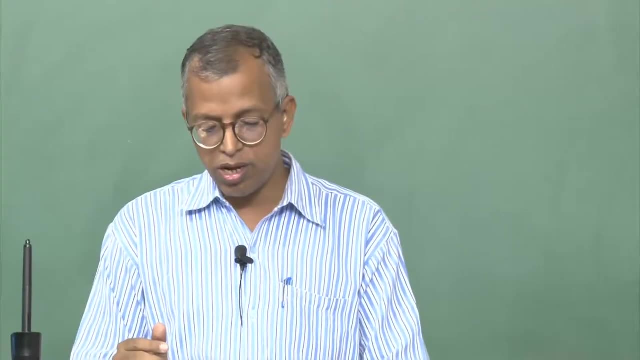 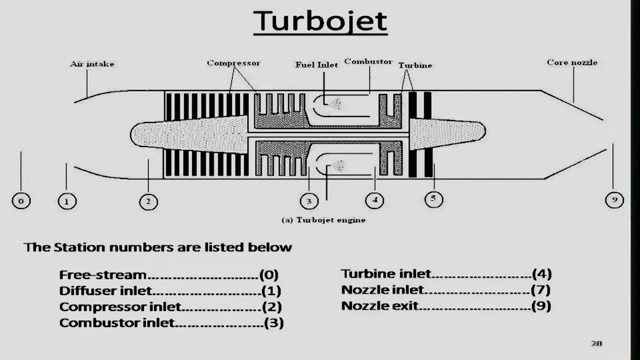 itself right. So you need to have auxiliary. in order to overcome that, one can think of using a compression. and when you talk about the compression you know because it has to give some ram pressure to make it. So for that reason we need to have add also turbine. So a turbo jet engine is. look at 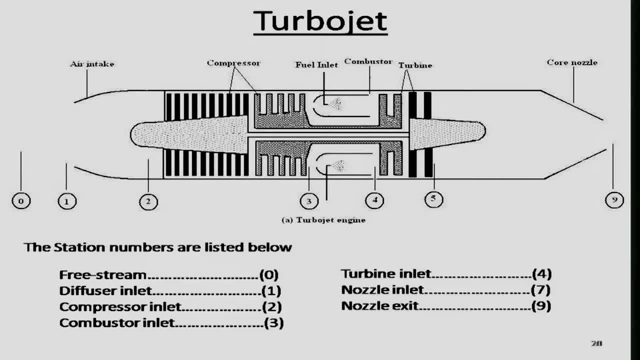 it is nothing but similar to the ramjet engine with a turbo machinery. if look at, there is a compression and to run the compression we need the turbine. keep in mind that the work obtained by the turbine You just mean to the run the compression, that is the turbo jet engine and all the thrust. 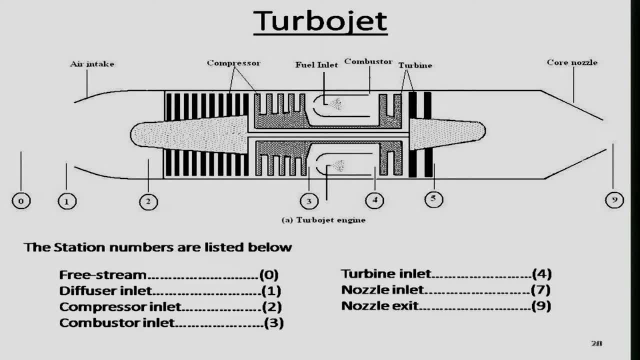 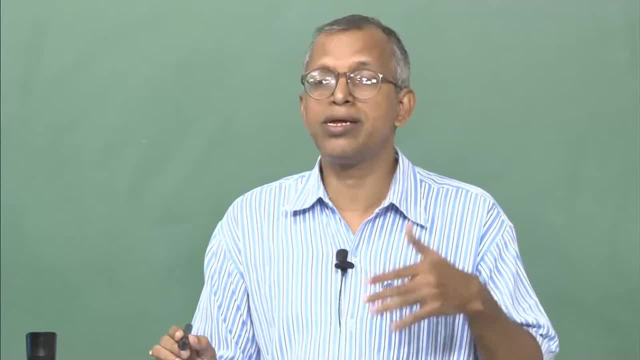 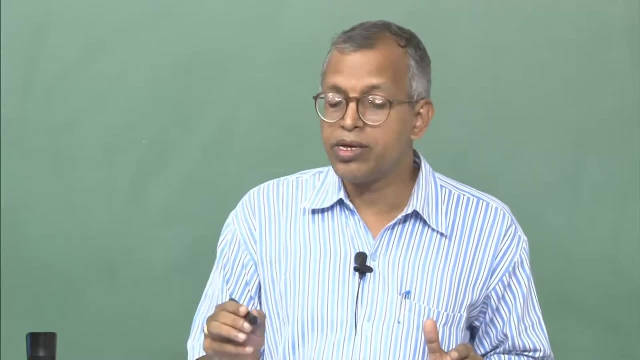 is being produced by expanding the gas in a nozzle. that means, in case of turbo jet engine, the thrust is produced by expansion of gas in a nozzle. rather, nozzle is the component which gives you the thrust, not the turbine or the compressor right. So this is the very 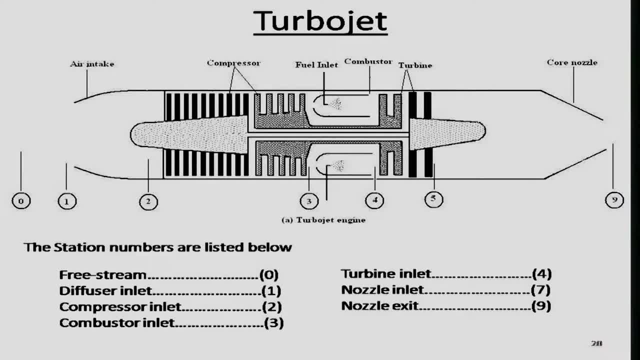 important concept you should keep in mind, unlike the other, So we will be using this station numbers like 0 to 2 is your air intake and 2 to 3 is your compression, 3 to 4 is your combustion chamber or combustor, and 4 to 5 is your turbine. 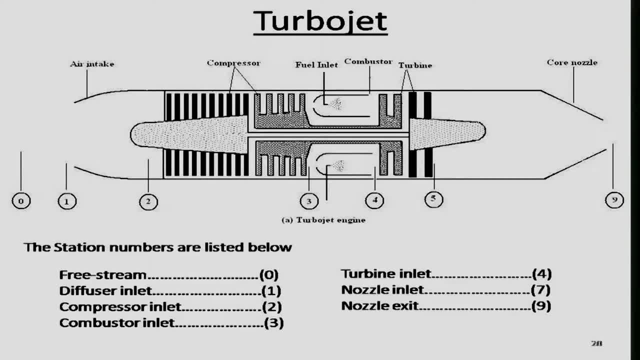 that is expansion, and 5 to 9 is your, what you call, of course, 5 to 6, and you know 7. you can say there will be 7, this is known as the jet pipe, but, however, 7 to 9 is the. 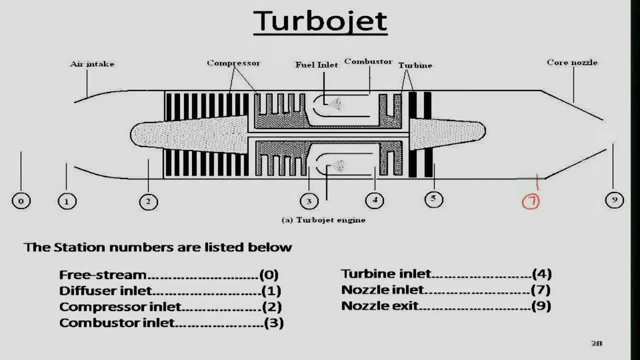 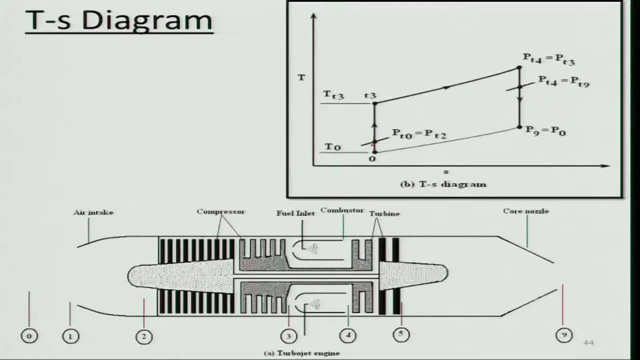 nozzle right. So I have already discussed about this thing. now we will be what you call looking at how the processes you know in a T S diagram. So if you look at, this process is basically what you call compression- compression in air intake and this is your compression. 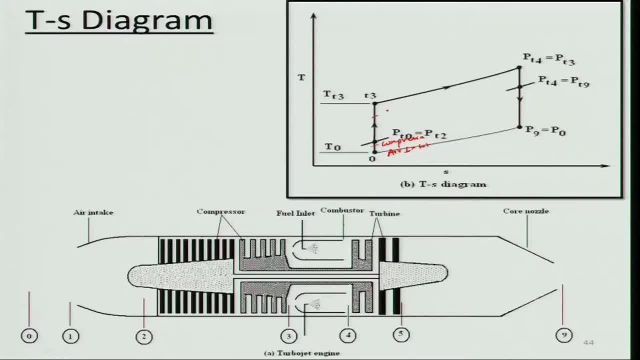 . . . . . .� So, this is the combustion or the air intake right and these is your combustion chamber constant pressure and heat addition. And this portion is your expansion in a nozzle sorry expansion in turbine and this is in your nozzle right expansion. 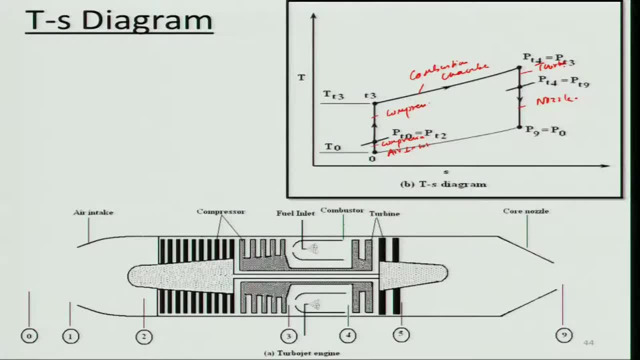 only thing you are having a contribution from compression and a turbine, that is all. but it is similar and if you look at p v diagram, it will be similar to that, only the division will be there in the compression and expansion part. 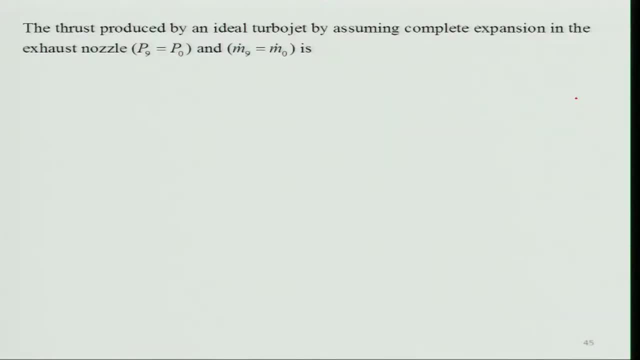 So now what we will do. we will do the similar, you know methodology to derive the expression for the thrust that will be for an ideal turbojet engine will be same that what we have derived, that m dot 9 v 9 minus m naught v naught, If I take this a naught out you. 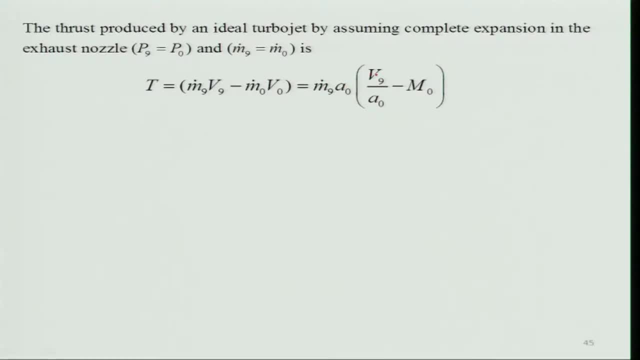 know, and m naught 9 out, I will get v 9 by a naught minus m naught. m naught is the type method, So a naught is the speed of sound and we have already know this thing. And the specific thrust can be, you know, defined as I told earlier, the thrust divided by mass. 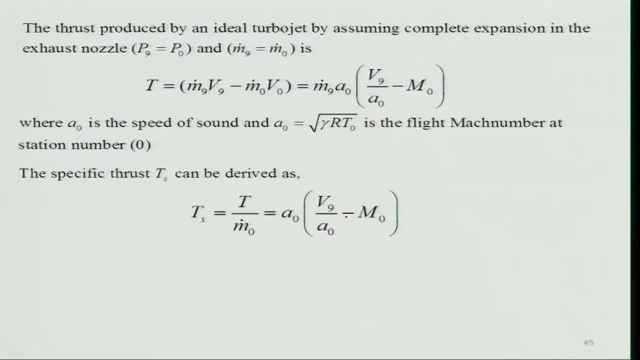 flow rate of air is nothing. a naught v 9 by a naught minus m naught, The same thing. what we have done, So space, and we know that v 9 by a naught square is nothing but a 9 square. 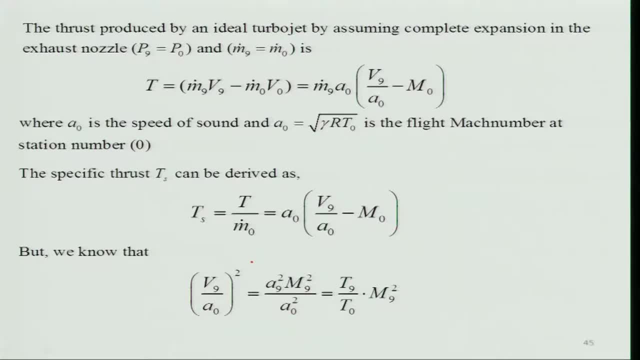 m 9 square and a naught 9. we know that it is gamma 9 r 9.. So this is cancel it out. gamma is same as that. So you land in getting t 9 by t naught into m 9 square. So what we will be doing, we will be doing the similar stuff of relating. 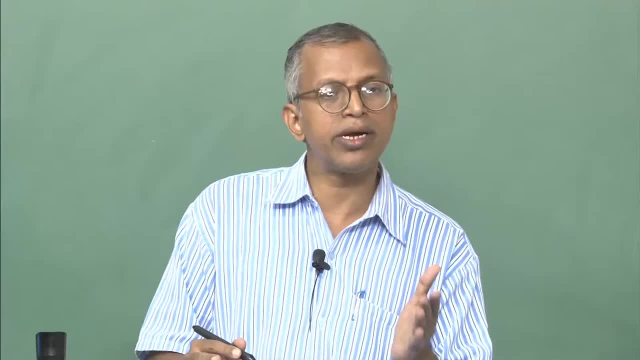 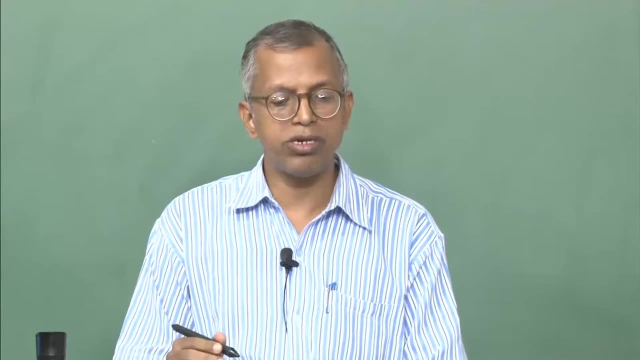 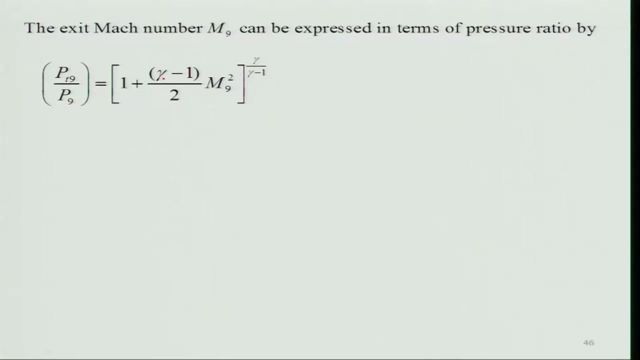 the various, you know, pressure and temperature parameters in each component. It is just extension of what we had done for the So p t 9 by p, you know 9. we know that it can be expressed for isentropic flow in terms of Mach number and exit Mach number. if I just rewrite back that it will be m 9. square is. 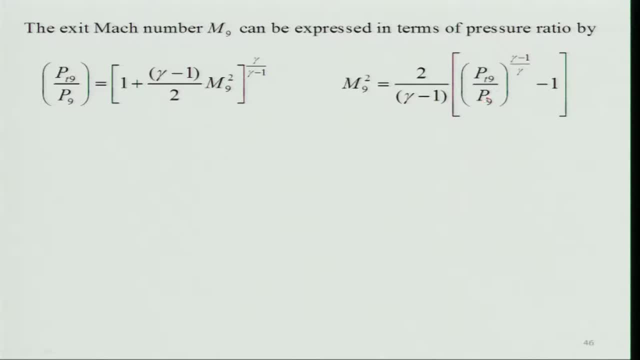 equal to by gamma minus 1 p t 9 by p 9 power to the gamma minus 1 divided by gamma minus 1 right. So we will be looking at this p t 9 by p 9.. And look at the various pressure ratios. So, if you look at in the similar way- and I have 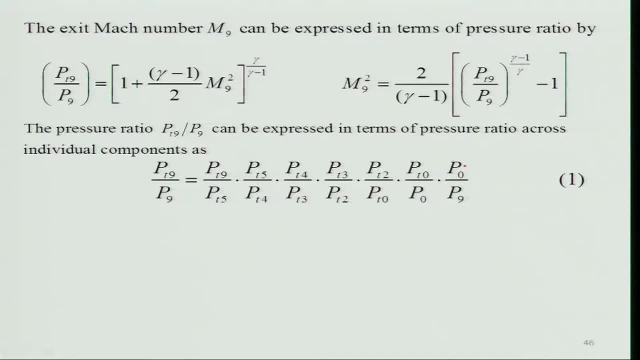 just written down here And if you look at it is a fully expanded. So this will be one and T? t by p? naught what it would be. this will be your pi? r and T? t by p? d. T 2 by p? t naught. this is nothing but your pi? d. 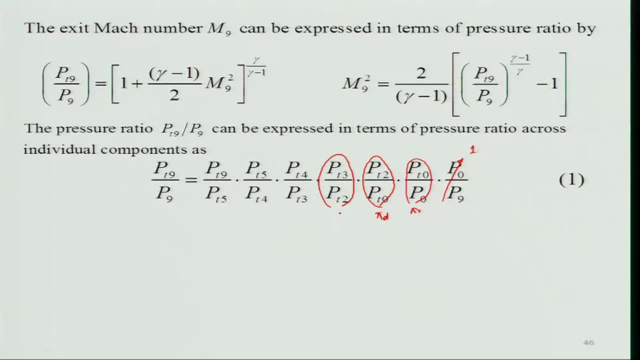 And this is P t by p naught. P t 3 by P t 2 is pi C and P t 4 by P t 3 is nothing but pi B, and P t 5 by P t 4 is your pi turbine. and this is your nozzle if you say: 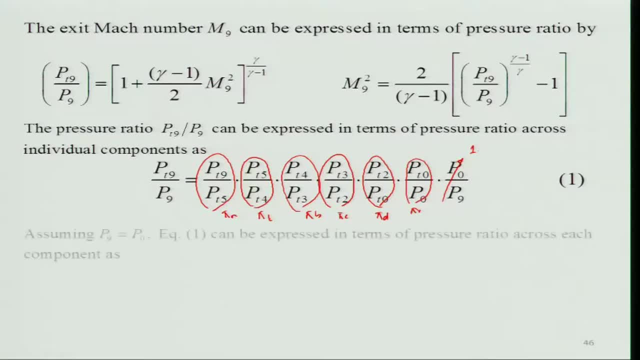 And we know that this what you call, and we can express in this, similar in terms of pressure ratios and under ideal condition, what we can say. we can say that pi B is equal to 1, yes or no? and what happens to your turbine? pi t, can I say 1.. 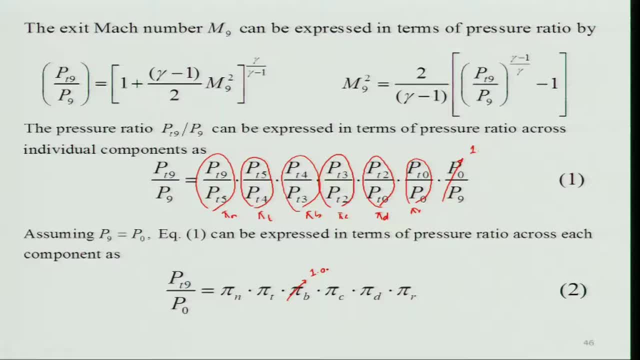 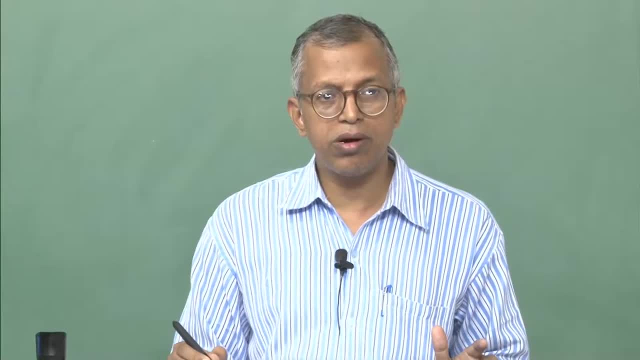 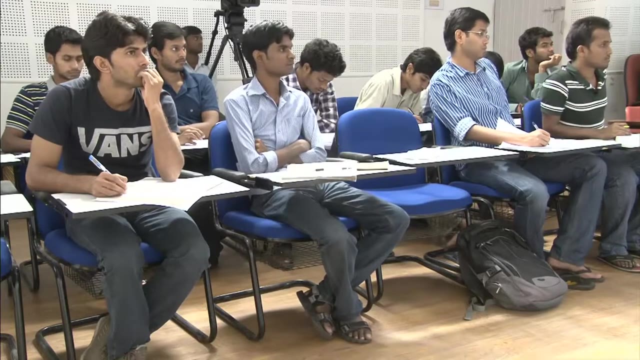 I see I can say 1.. No, sir, No, no, right. and pi d, can I say 1, yes or no? Total pressure ratio: what happens in the pi d Acrose compressor? no, No. compressor, no, turbine is no, that, as you were saying, right, because we are, you know. 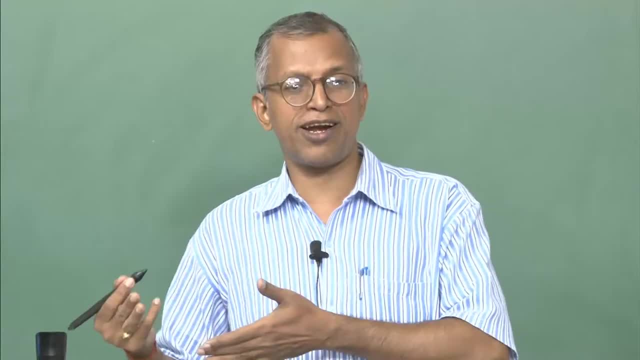 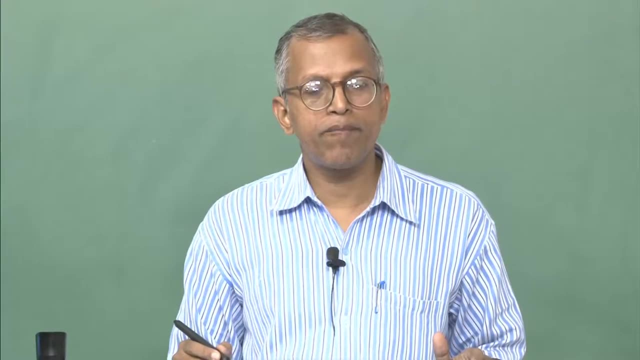 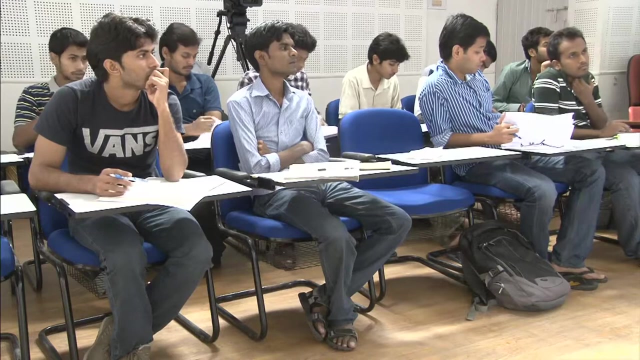 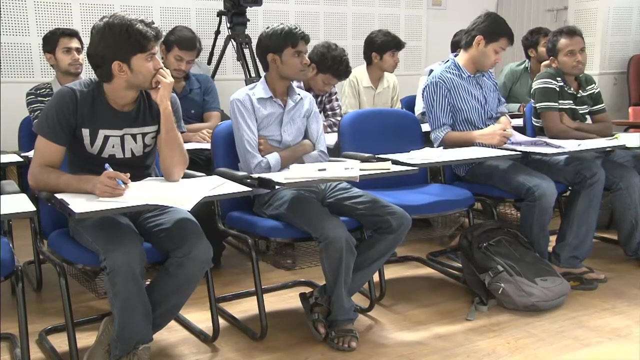 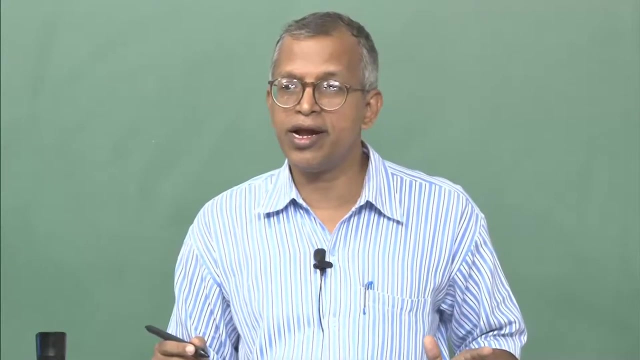 getting something, doing the work on it and extracting the work in the turbine, right. So what about pi d? what we did in the ramjet engine? total pressure. what is happening? Ram pressure, Ram pressure will be what total pressure will be, remaining same or it will be depend. this is isentropic process, right? 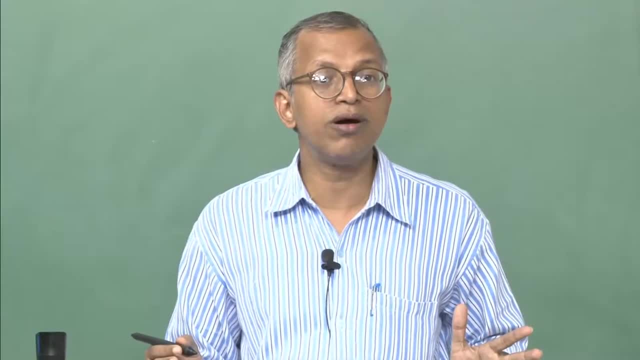 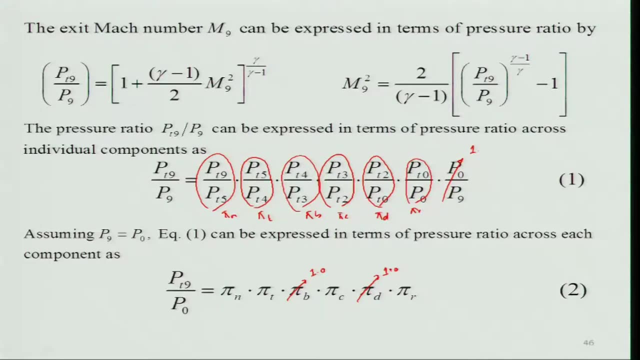 One, One right, yes or no? Yes, Yes. So, and what about nozzle One? It is also one right, because we are just converting, you know, kinetic energy into the where, into the static pressure, or the dynamic head, to the static head in case of your air intake. 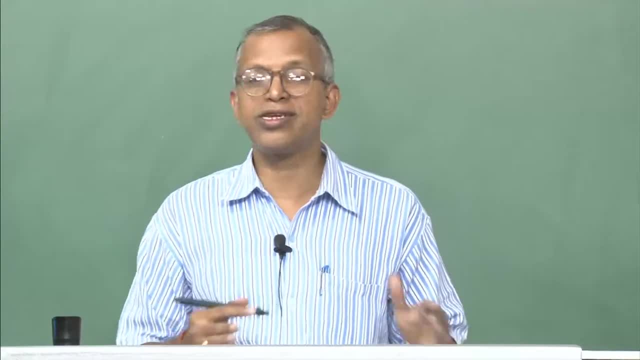 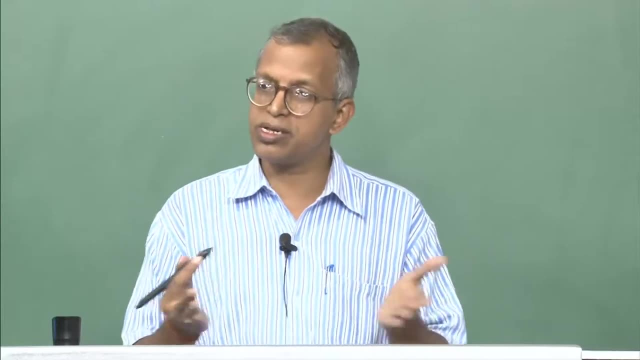 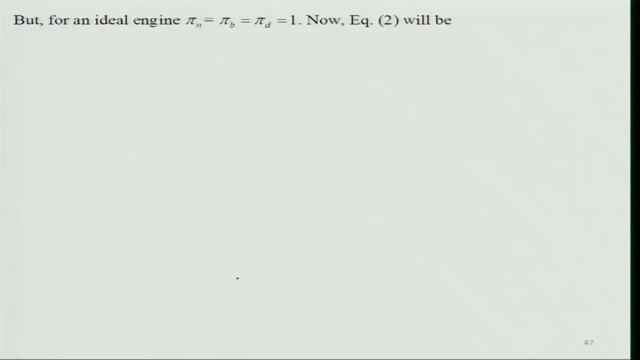 and this is other way around the nozzle, just opposite the static, you know, like static pressure, we are converting, Yes, We are converting- to the dynamic head right, but the total pressure is remaining constant. So therefore, you will have to be, you know, understand this concept. So pi n, pi b and 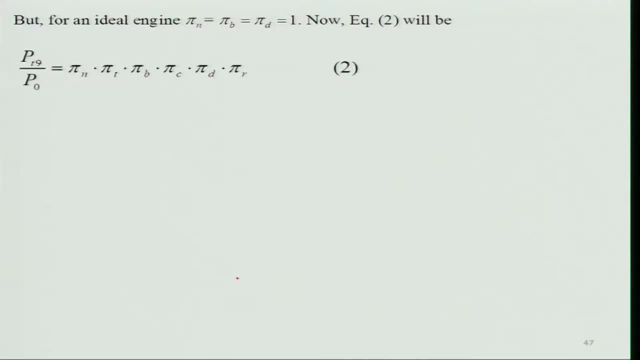 pi d is equal to 1.. So this equation becomes, you know, like p t by p, 9 pi t, pi c, pi r. in case of ramjet engine, pi t is equal to 1 pi c, because there is no compressor, no turbine. So you: 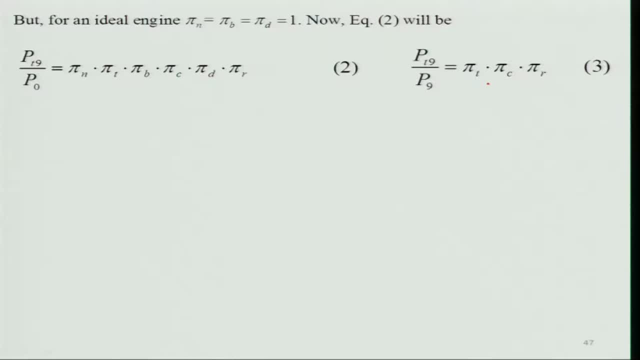 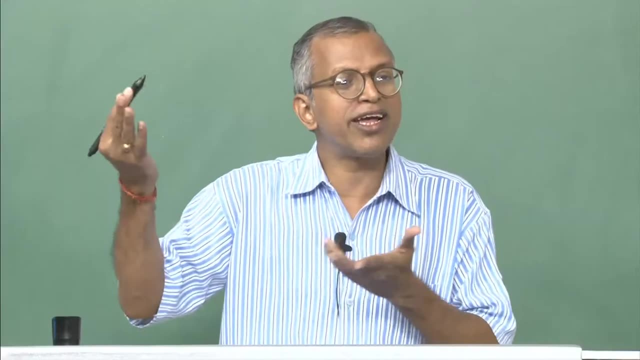 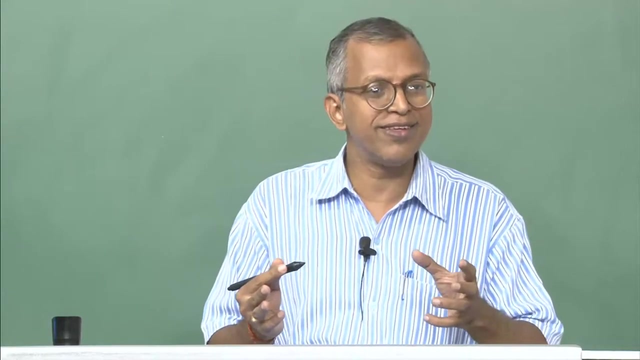 can directly get this expression. that means if I know this equation, you know expression, I will get ramjet, turbojet, just making some parameter one, you know. that is why that is the beauty of this analysis. right, I need not to do anything If I say pi t, pi c is equal. 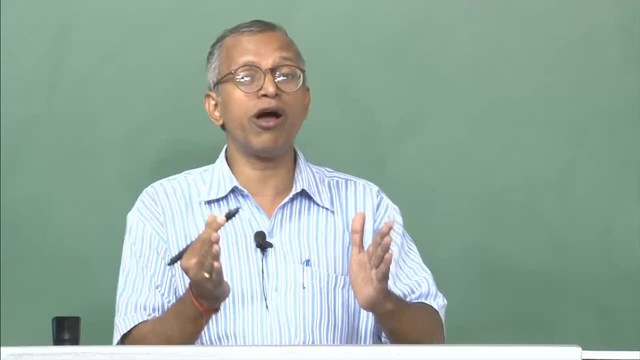 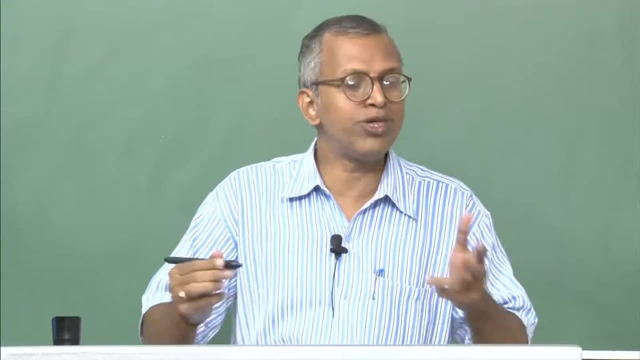 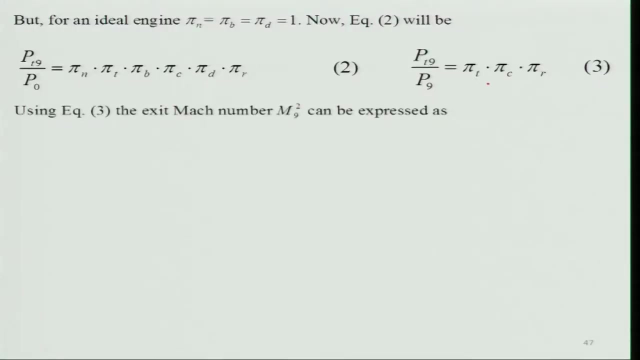 to 1. that means it is a ramjet engine, right? that is the beauty of this relationship, where computer you can do very easily, I can put a condition and do that, ramjet, scramjet, same equation you know, So that you should must appreciate of this relationship and a using equation 3: exit Mach. 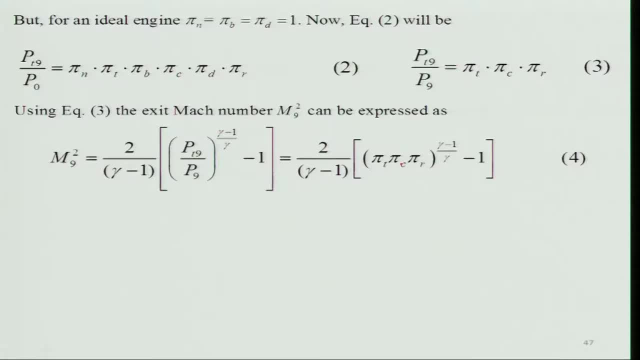 number I can get because I have already derived. that is nothing but same as that. and except this, you know pi t and pi c being coming to as compared to the ramjet engine, right? So if you look at this similar to that, what we have done for the ramjet, only two terms have 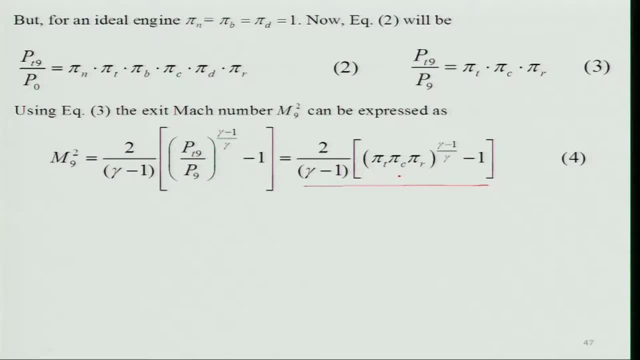 come for the turbojet pi t and pi c. So where, as a pi r you know is, we can relate to the tau r gamma power to the gamma minus 1, and similarly for pi c and pi t. these are isentropic relationship. pi means it is a pressure. 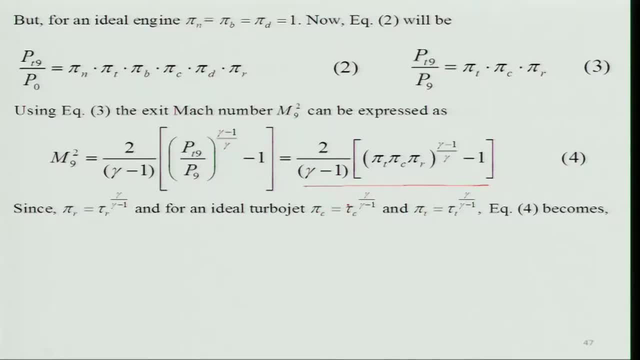 ratio. tau means it is the temperature ratio, So we know the pressure ratio can be related to the temperature ratio with the help of this gamma. you know of the index, So you know square, you can write down here itself. if I put this values over in this place you. 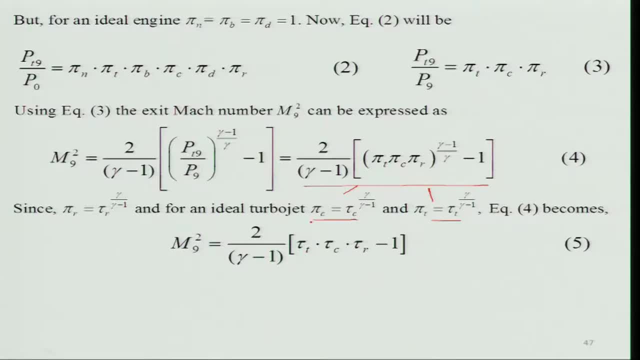 know. and also for pi, r I can get instead of pi, I can get in terms of tau, that is tau t, tau, c, tau r, right? So we will do the similar way of getting this t 9 and t 8.. So we will. 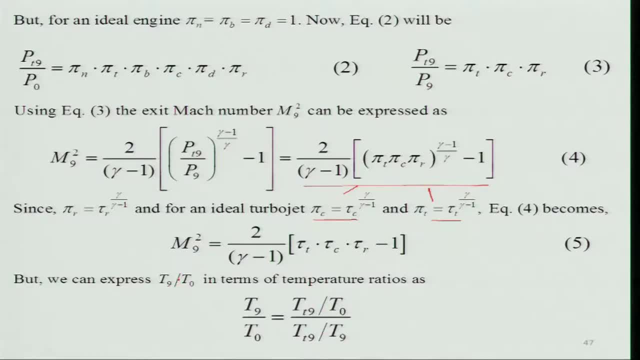 do the similar way of getting this: t 9 and t 8.. So we will do the similar way of getting this: t 9 and t 8.. So we can write down t 9 by t naught. we can write down t t 9 by t naught, divided by: 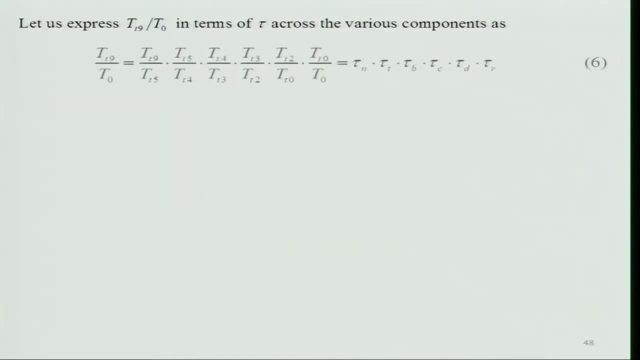 t, t 9 by t 9 and we will go on doing that. all those things, if you look at it will be. you will get this: tau n, tau t, tau b, tau c, tau d and tau r. If you look at, tau d is what. 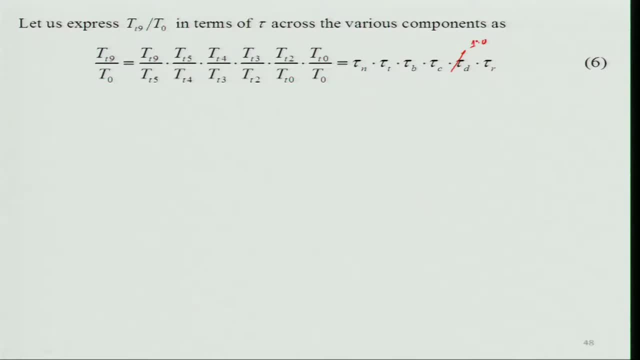 is it one? because this is adiabatic process. in the air intake, there is no heat, is there? So therefore that will be one. similarly, in the nozzle, is it? you are adding some heat, you cannot, you are not doing anything, So therefore it will be one. So what about? 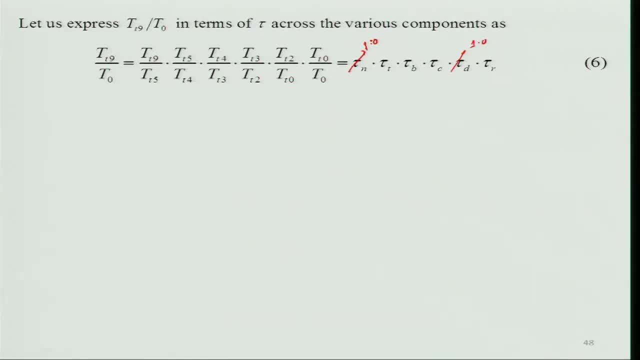 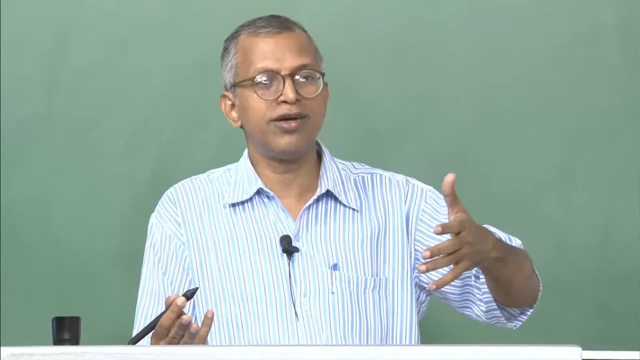 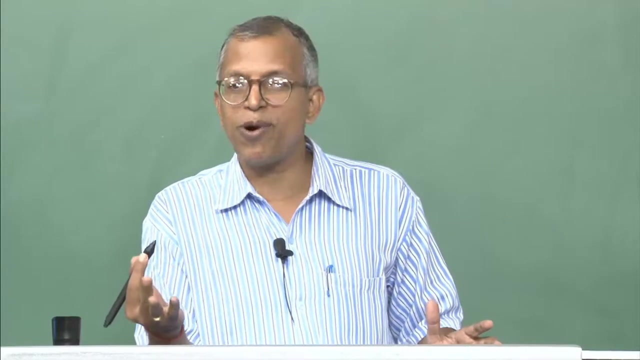 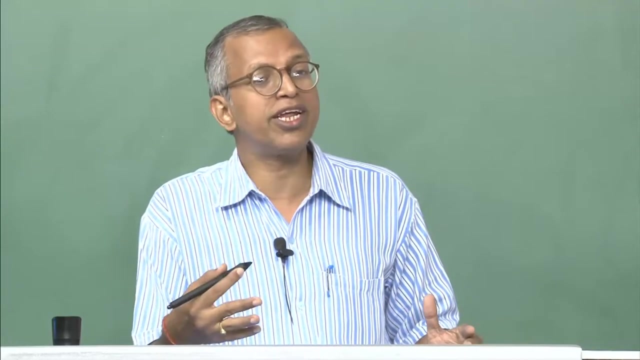 tau c and tau t. can I make it one and tau b? certainly know, because I am adding some amount of heat, right? can I make it? I cannot make the tau t and tau c as one. that means the total temperature across the compressor and across the turbine are changing, So it. 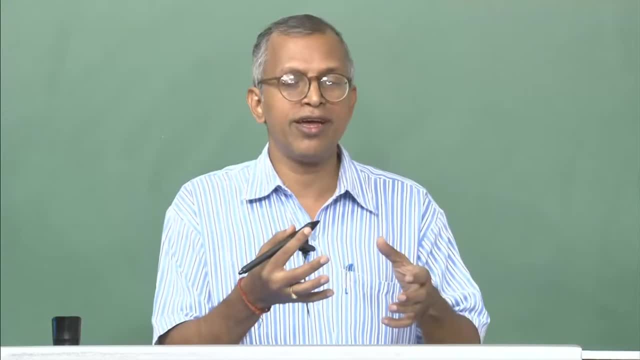 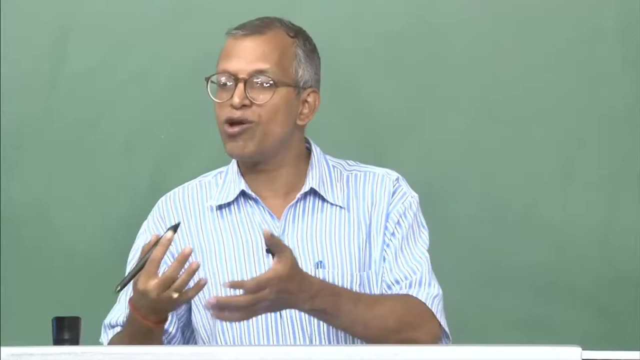 cannot be one, because in one case, compressor, you are giving you know amount of work and in that turbine you are extracting the work from the fluid, So there will be change in total temperature. otherwise you where you will get anything. So therefore you cannot. 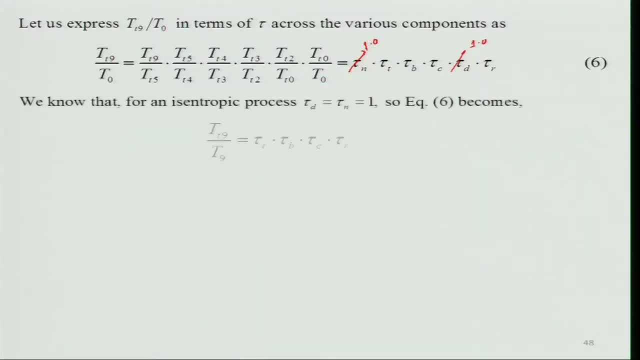 really make it one. So t t 9 by t naught it will be tau t, tau b, tau c, tau d and tau r. So we can write down: tau t by t naught divided by tau t, tau b, tau c, tau d and tau r. So we can write down: 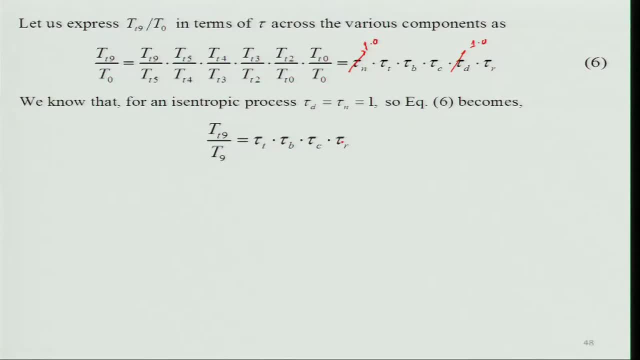 tau t by t, naught divided by tau c, tau b, tau c, tau d. and again you can say this here, you can appreciate this point that tau c and tau t will be one, in case of. I am getting right the same thing, I am repeating So that it will enter into your mind. So the expression: 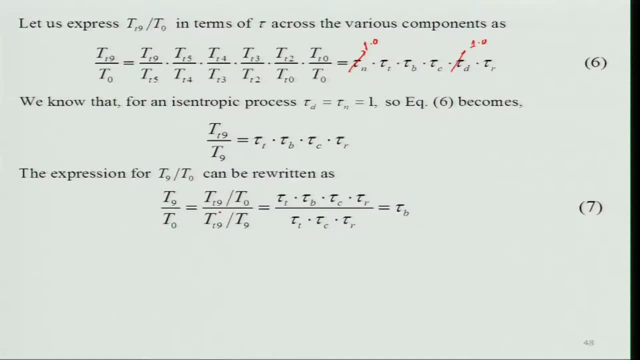 t 9 by t naught can be. really, if you look at it is interesting. if I put this t t 9 by t naught, all those things this is can, and also t t 9 by t 9, you will see that it is. 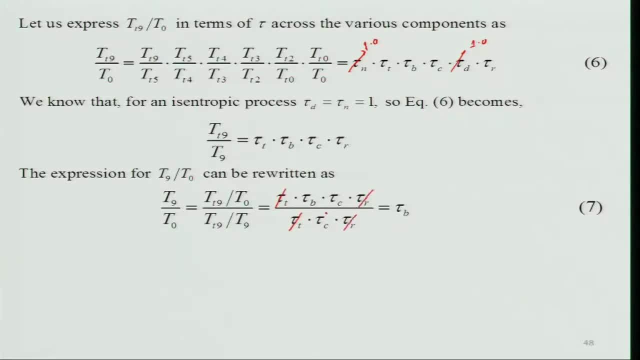 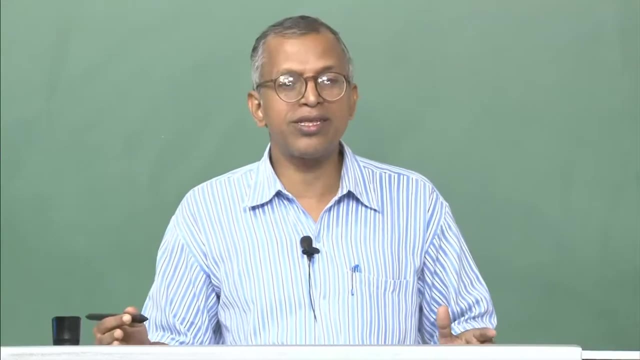 can be cancel it. So this can be cancel it out. this can be cancel it out. and the tau c can be cancel it out. it happens to be tau b and what we had seen in case of your ramjet engine, yes or no? we are doing the same thing but making a little complex. but this is cancel it out. 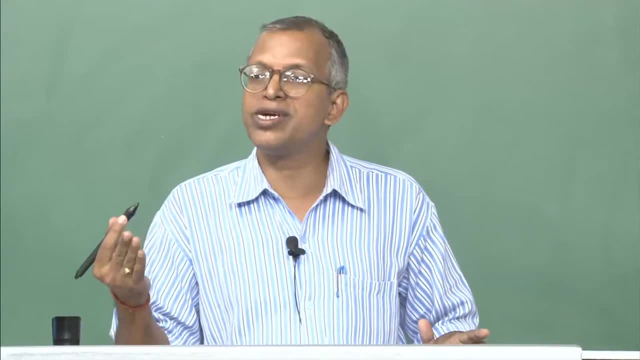 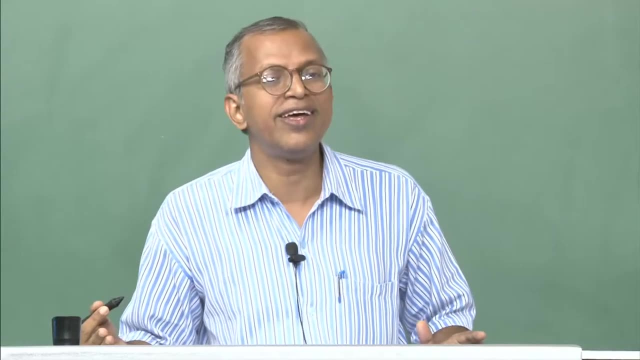 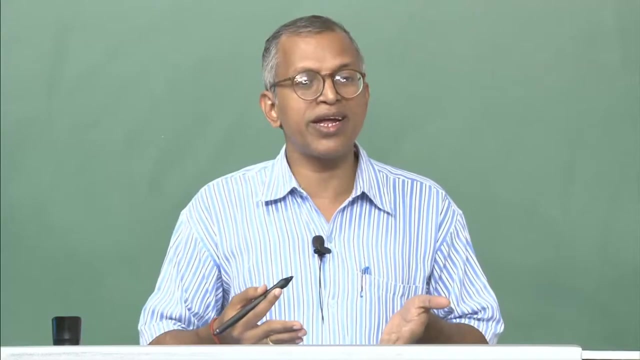 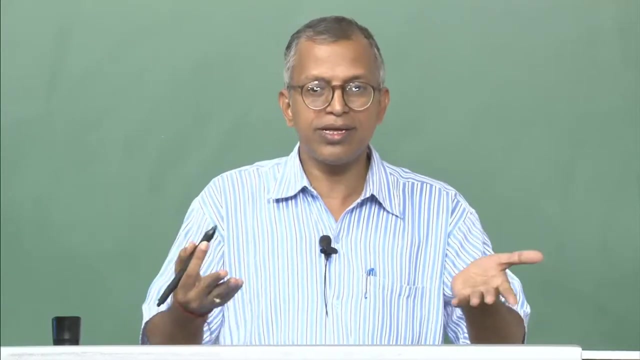 which is obvious, because the turbo in the turbojet engine, the work, you know hardness, by the turbine. So this is being utilized by the compression. therefore it must be t, 9 by t, naught will be tau b. it will be how much it added into the combustors. right, that is the thing, what? 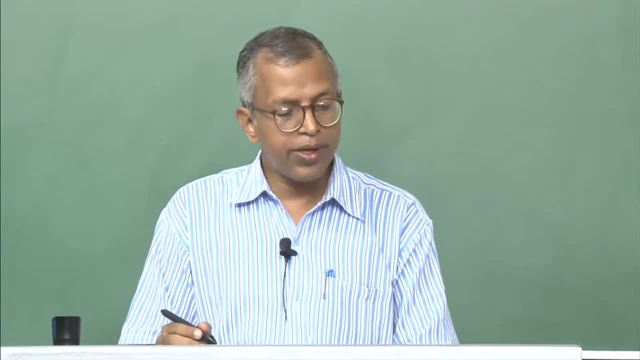 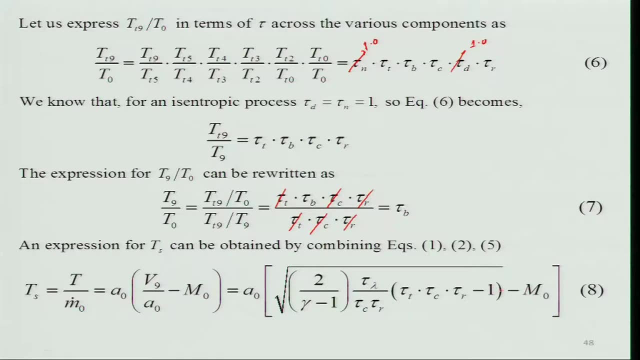 is saying, and this is true also ramjet, So the t s. you can just substitute these values, v 9 by v, naught right, and you will get a expression which looks to be little frightening, but however, it is quite simple. So I am not expecting that you should remember this expression, but however, you must know. 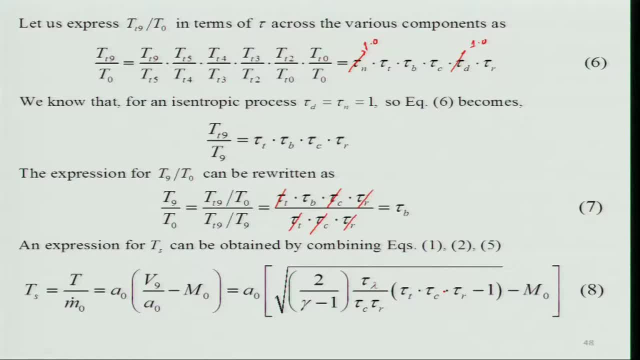 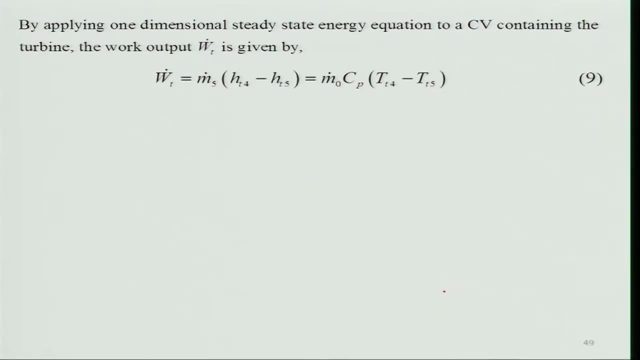 how to go about or to derive it. that is expected right. So, and which will be quite simple to derive, this expression and very important, we need to now relate this turbine work into the compression work, because we will have to get relations, So let us see, between the compression and turbine, So we will assume the one dimensional. 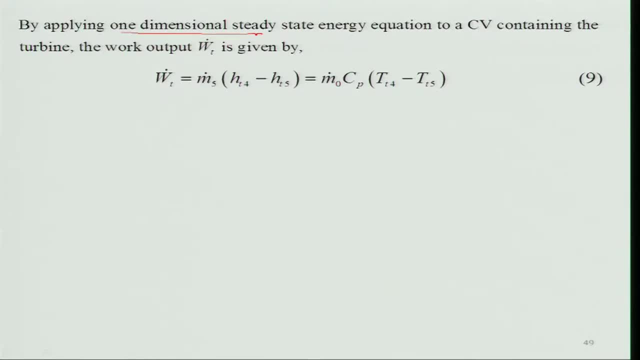 steady state energy equation. you know this thing and we will apply this to energy equation. control volume and the turbine work will be: m dot 5 is equal to s t 5 minus s t 5 right, because the right in the turbine- and you keep in mind that here we are assuming you know- 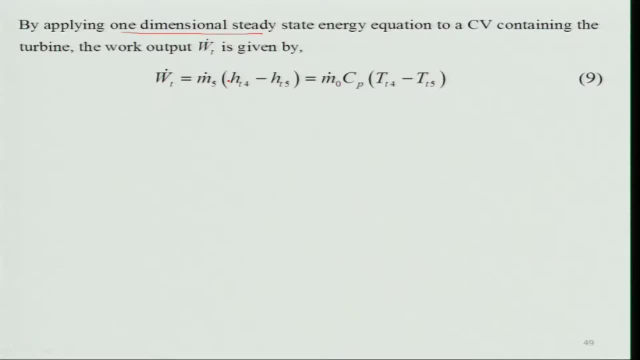 like the mass is. So the mass is maintained because one dimensional flow we are talking about. So m naught 5 is equal to m naught 4. you are not adding anything except you know. So same fluid is going. so 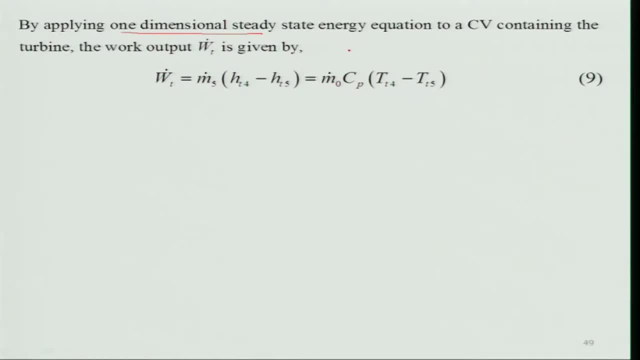 therefore, which is nothing but that m naught not keep in mind that here I am saying it is very, very less than m naught 5, or is very, very less than m naught. So therefore I am saying this is m naught is equal to m naught 5.. 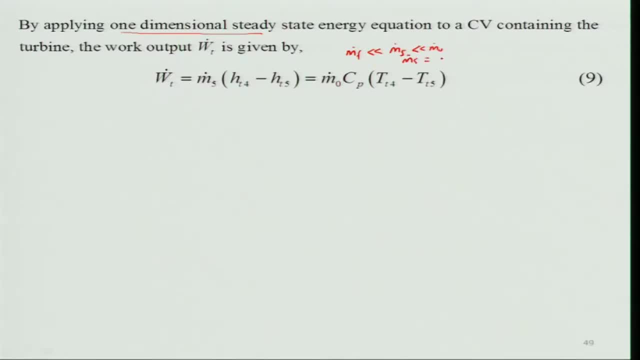 m naught 5 is equal to m naught plus m naught F, right, but I am assuming this. So therefore m naught F C p, T t 4 minus T t 5. similarly, I can have a compression which is same as: 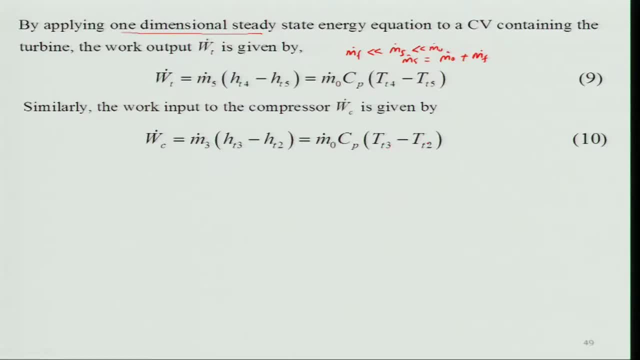 that m naught C p T 3 minus T t 2 right. and when we equate this, the work done by the turbine Claus, которых M 0 F, c p T 3 minus T t 2, by using one dimensional steeping All the 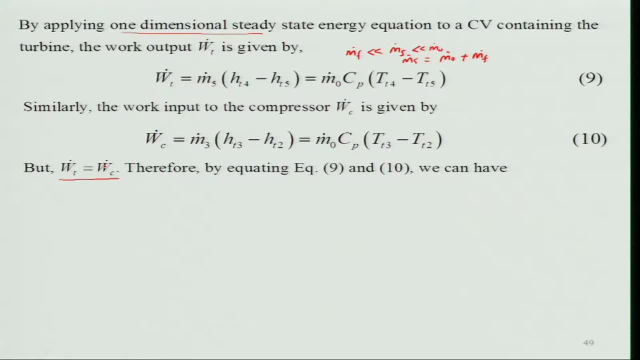 turbine is same as that as the work, you know, taken by the compressor. then we will get an expression you know: tau t is equal to 1 minus tau r by tau lambda in the bracket tau c minus 1.. Keep in mind that we can express in terms of tau lambda, because that is a thing. 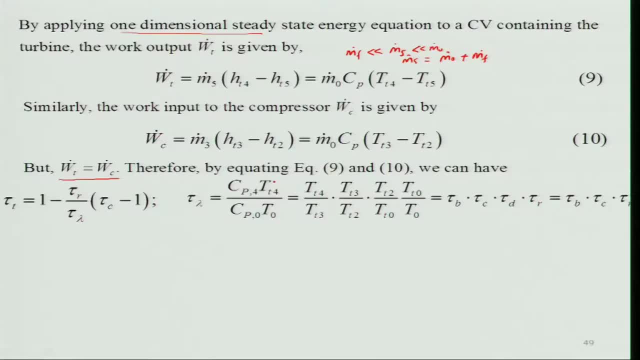 how much heat you know being added, or the total enthalpy at the exit of the combustor divided by the amount of enthalpy is entering into the engine, right? So if you look at it, is you know you can rewrite it because this will cancel it out. t t 4 by. 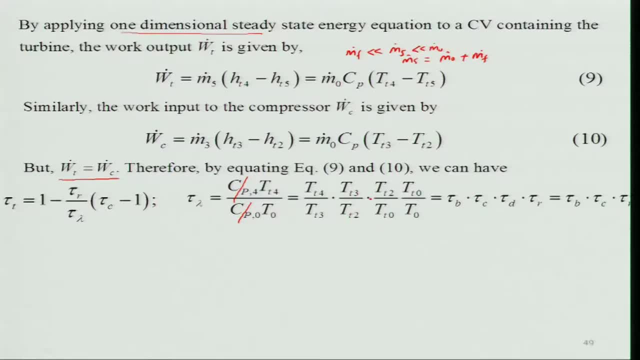 t t 3 into t t by t t 2 into t 2 by t t naught and t t naught by t. So you can write down in terms of all this: tau b, tau c, this is the compressor and tau d, this was the air intake. 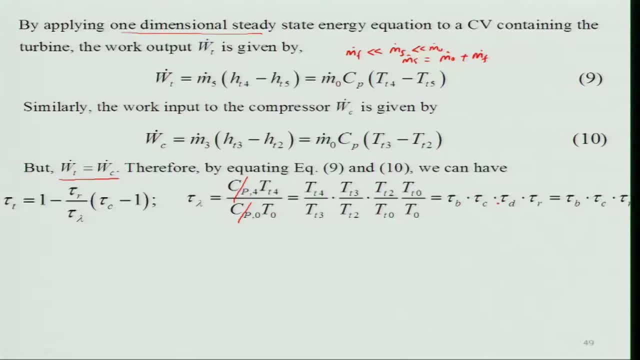 and tau r And you know that tau d is equal to 1 and right because of it is adiabatic process. we are saying no heat is going out, but in real situation it cannot be. but ideal under ideal system is okay. So the fuel air ratio can be expressed in terms of known variables as 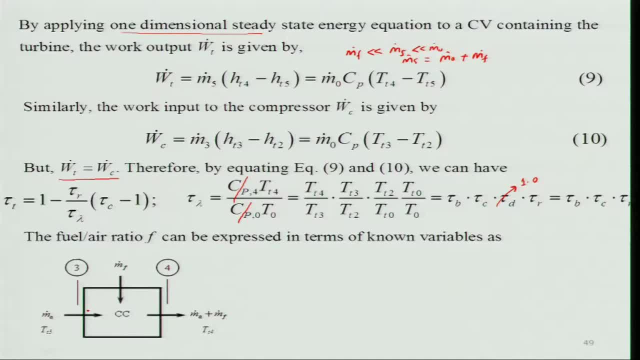 you know, we will have to consider this combustance, which we had done similar thing in case of a. So we can write down m dot f divided by m dot a, nothing but c, p, t, naught, delta s, c, which you will see that tau b, tau r tau c minus tau r tau c. this is some step I have omitted. 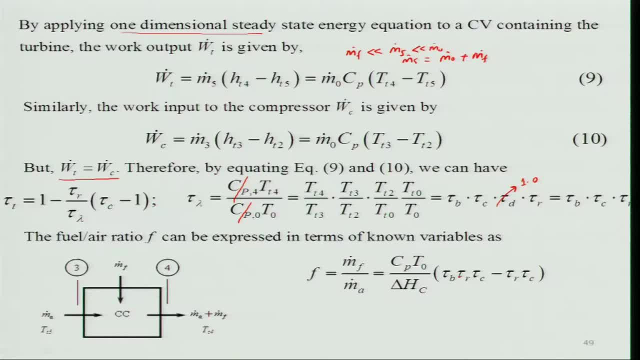 here. but you can do very easily and in case you will find some problem, you let me know. right, And t, s, f, c, you can get very easily. that is right. That is f divided by specific thrust, right, and you will put this values. you know now. 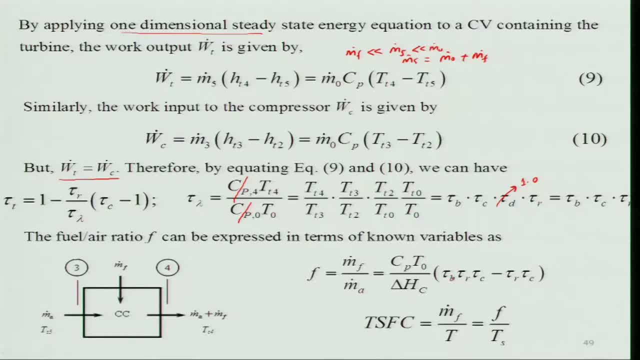 we are having. several terminologies are coming, like several ratio, temperature ratio or pressure ratio. keep in mind that we can, you know, change this tau c in terms of pressure ratio of compressor. similarly, tau t, we can, you know, some places, wherever it is required, we can change into. 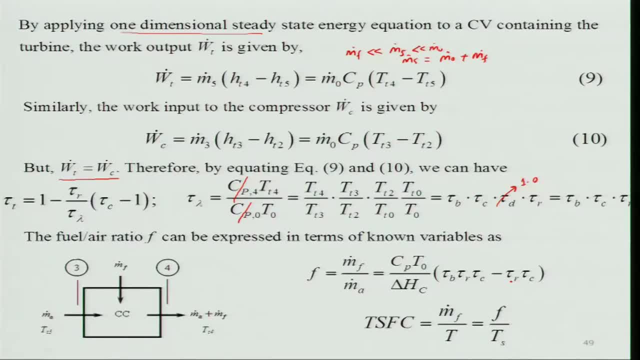 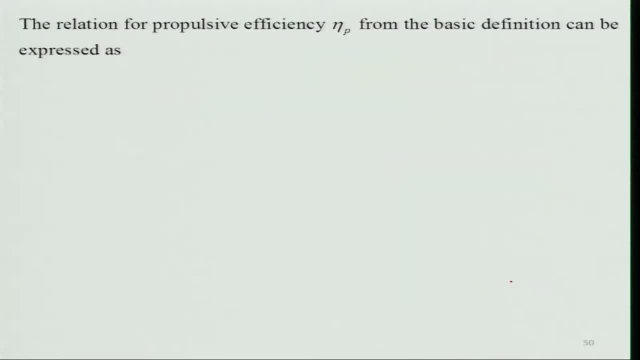 the pressure ratio across the turbine right, and using the isentropic relationship, So the relationship for propulsive efficiency, we can write down 2 t v, basically the thrust power divided by kinetic energy change in the engine, that is, m dot v, 9 square minus. 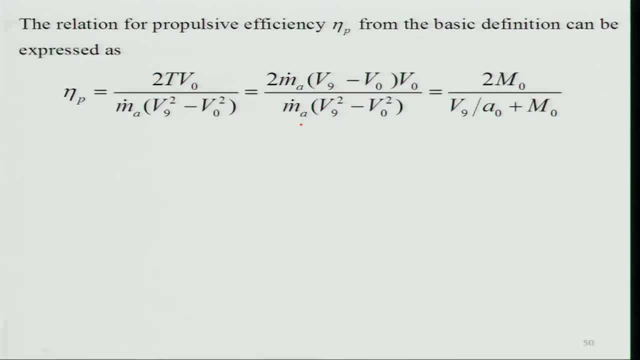 v naught square divided by 2.. If I just you know, write down the pressure ratio across the turbine right in in place of thrust, this expression m dot a into v 9 minus v naught, you will see that I can cancel it out, and this will cancel it out and I will get v 9. 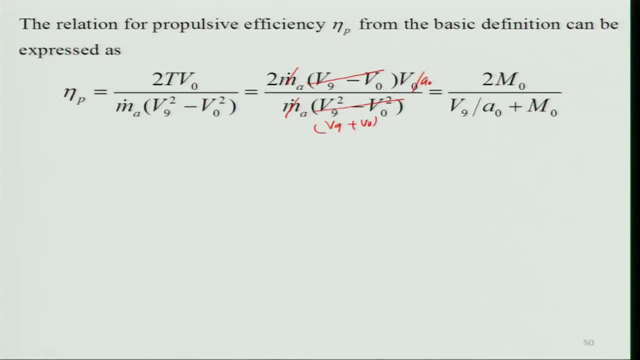 plus v naught. right, If I divided by a naught square here and similarly a naught square here, I will get 2 Mach num, type Mach number divided by v 9 by v naught plus m naught. So this is the easier way of saying that because I know expression v 9 by a naught. 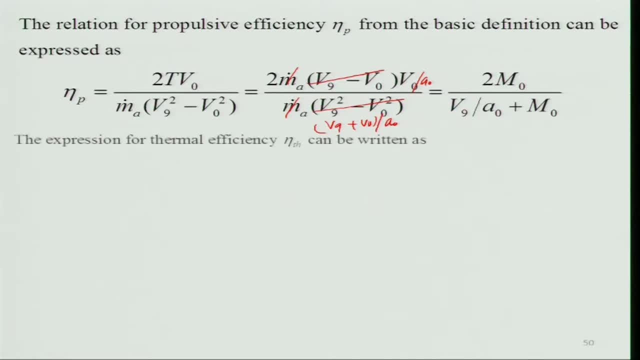 I can do very easily, right, And also you can see that how this Mach number is really affecting your propulsive efficiency and thermal efficiency. you can get, you know. do all those things, algebra, and you will get 1 minus divided by tau or tau c. keep in mind that here tau c has come. 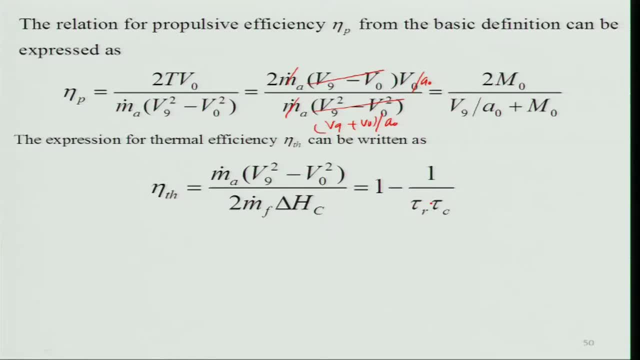 into picture in case of turbo jet right. Earlier it was 1 minus divided by tau or tau c right. So this is the easier way of saying that because I know expression v 9 by a naught I can do very easily right, And also you can see that how this Mach number is really affecting. 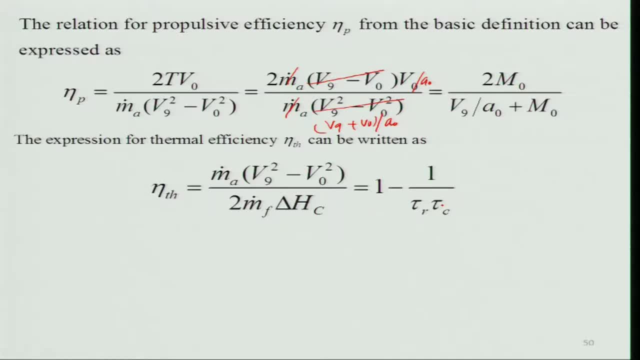 your propulsive efficiency and thermal efficiency. you can get. you know, do all those things algebra and you will get 1 minus divided by tau, or tau c is equal to 1, right in case of ramping. So prop overall efficiency will be nothing but propulsive efficiency multiplied by thermal. 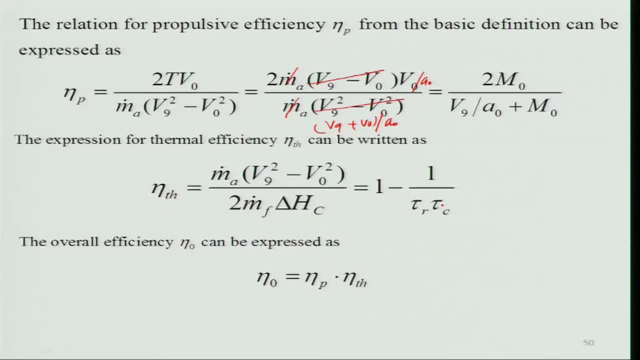 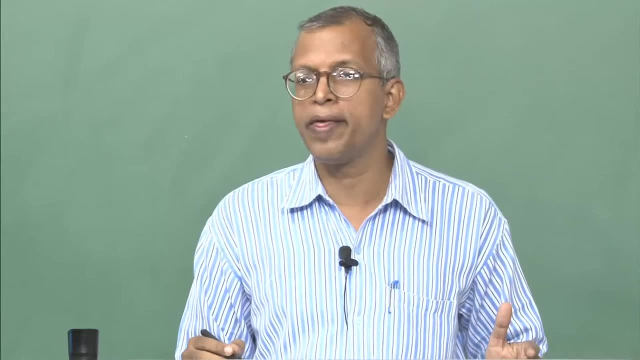 efficiency will be. that means by this we have derived all the expressions- we are armed with all the expression- to the carry out several metric studies. right, And just to summarize those, what have we have derived like? I will share with you the details of the app. We will have the values here. i will show you a few Here, what you will see. 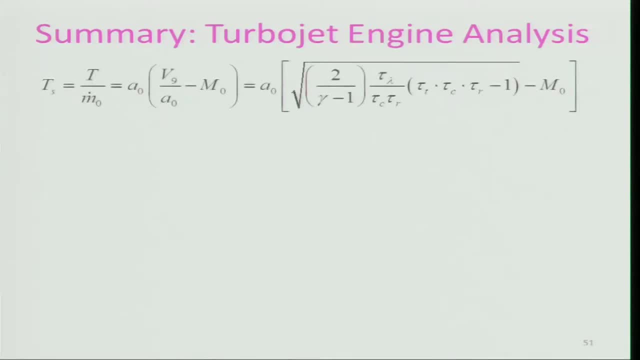 that is the specific thrust we have done and these are the expression, which is terms of various tau p, tau c, tau r, and we are using also tau lambda and in place of tau lambda. may be, you know this term: tau lambda, divided by tau c, tau r, is nothing but tau v some places. 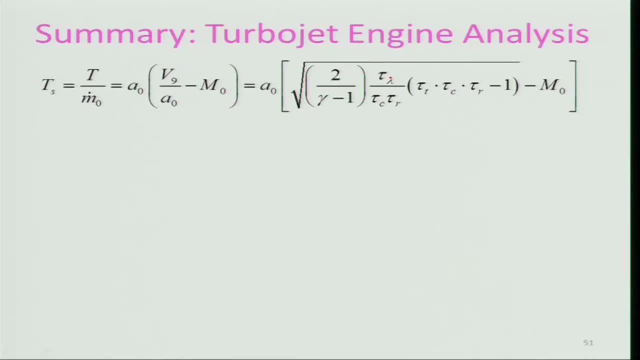 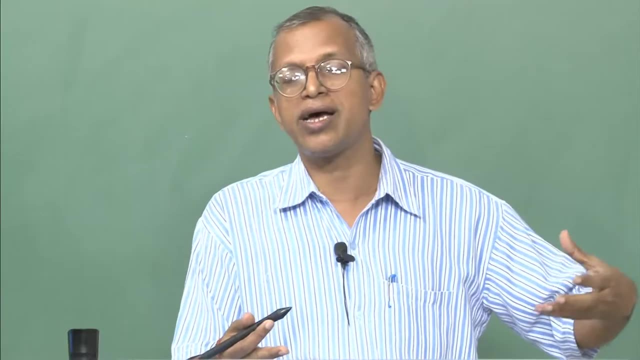 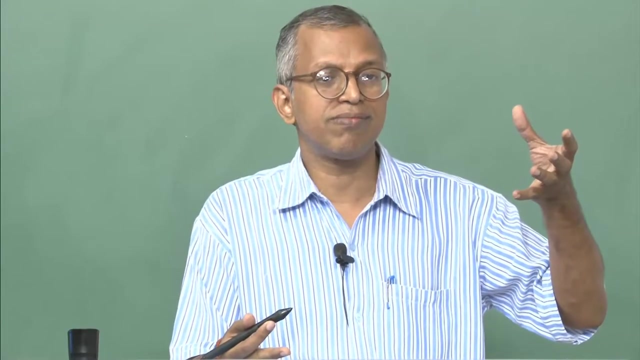 you can use tau v as well, right? So what is helping? this specific thrust expression is basically separating each parameters and it is arming with us, or helping with us, such that we can do a parametric studies that you must have. otherwise I need not to go for this. 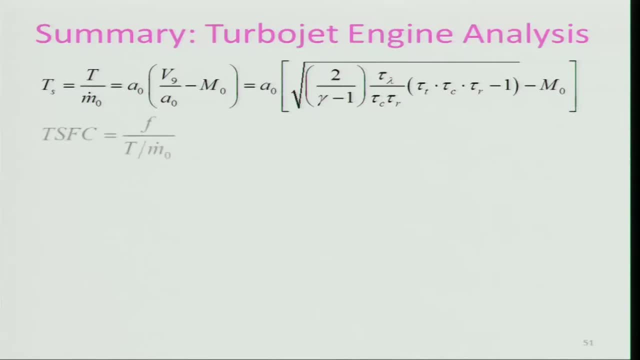 you know, unless I am not interested in parametric studies and which is essential when I am trying to understand, you know How it is. the performance is affected by the various parameters right, T, s, f, c, and we know that f is it can be expression in terms of tau p, tau r c, minus tau r, tau c and multiply. 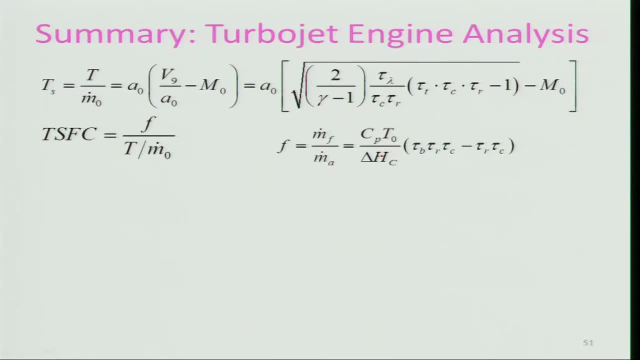 it by P, p, by delta x, And these are expression for propulsive efficiency, thermal efficiency, which we have discussed just now. and what we will do now, we will take along this system, which is called C r, which is a global thermalыл Sparking thermal efficiency. 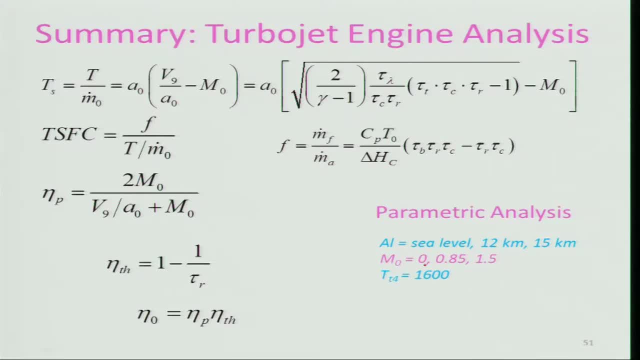 take three cases. One is the Mach number of zeal, that is, the sea level conditions, and another will take the long range, you know, vehicle or the aircraft. what we use: passenger aircraft 0.85 which can operate at 12 kilometers altitude, and then the fighter aircraft, which 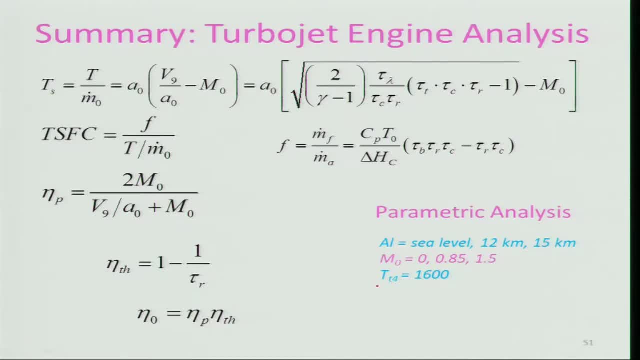 is responding to 1.5, 15 kilometer altitude And we are keeping this, the turbine, you know, like inlet temperature or the combustor exit temperature, 1600 Kelvin, right So, and what we will do now, what are the variables will be within, will be basically using the you. 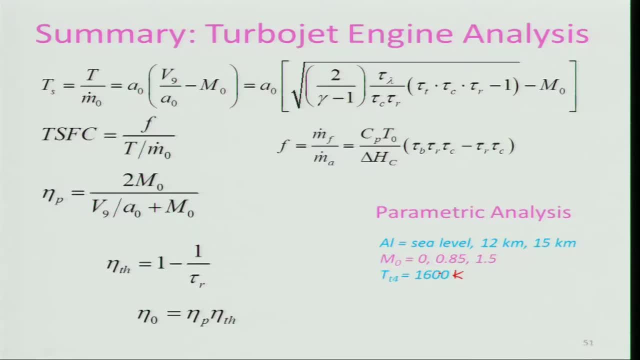 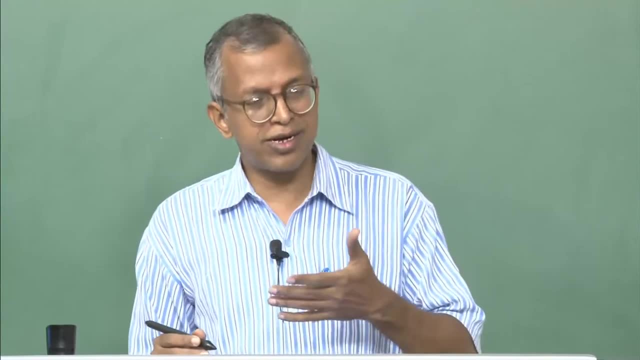 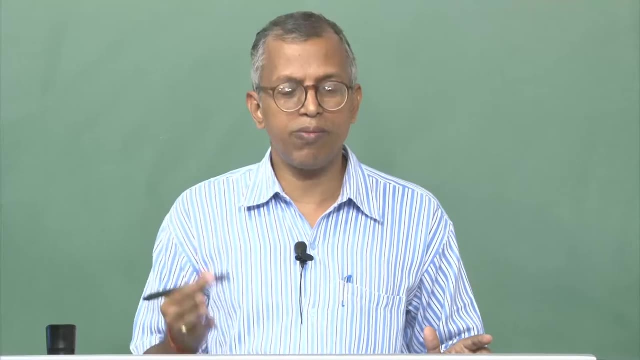 know we can vary this pressure ratio across the combustion. You can say that why not vary the pressure ratio across the turbine? you can do as well, because both are, you know, can be related easily with the work. you know, because the work, whatever you are getting from the turbine, is being utilized by the combustion. So generally 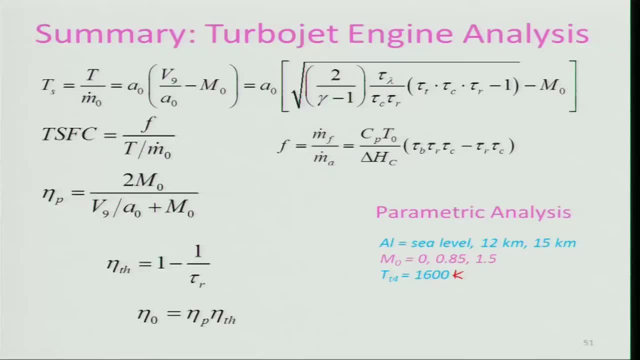 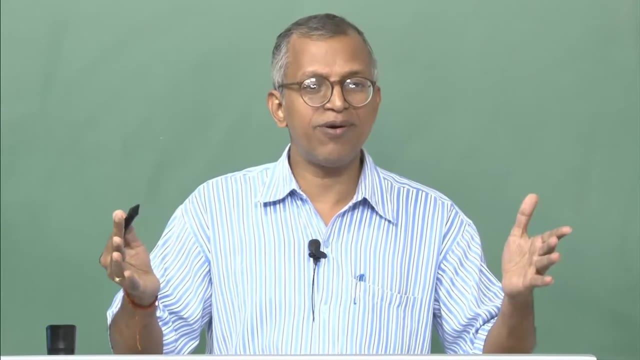 compression is a very important one. So, therefore, we use the compression as a parameter- that will be varying from 1 to hot, and see that how we can choose a compressor, how we can choose a you know pressure ratio, Because the compressor size and you know cost will be dependent on the pressure ratio- 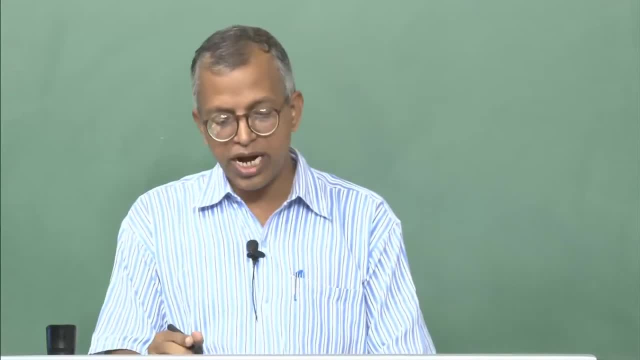 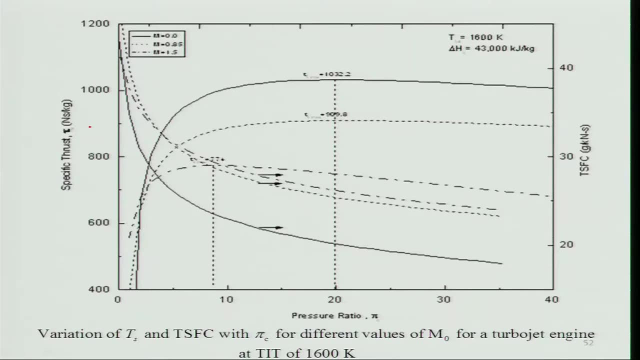 you are want to have for a engine right. So that is a very important one. So what we are looking at is the specific thrust right being plotted on the y axis and the pressure ratio plotted on the x axis for a turbojet engine which is having turbine inlet tension. 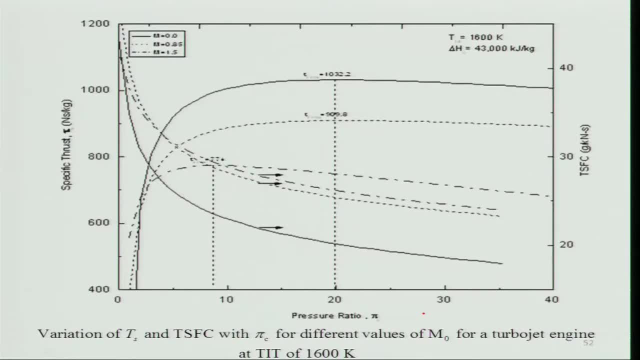 So this is a solid line. the specific thrust increases with the increase in pressure ratio across the compressor, and then it reaches the peak values here and then after that it decreases slowly, right? So what it indicates? that means there is a optimum value for the. 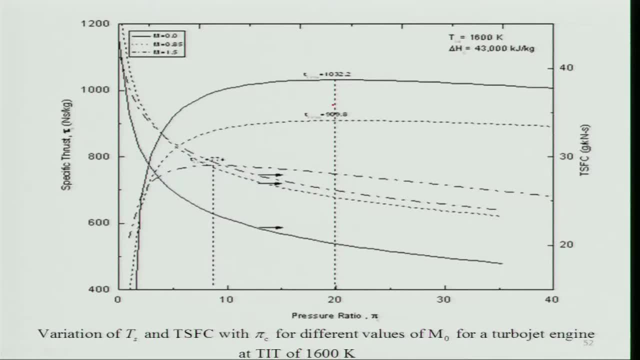 what you call Pressure ratio across the compressor, for which you will get the maximum specific thrust. and however, if you look at the T, S, F, C which I have shown here, that is, it is a very high values at the low, the pressure ratio of 1, you know, because we cannot have 0 pressure. 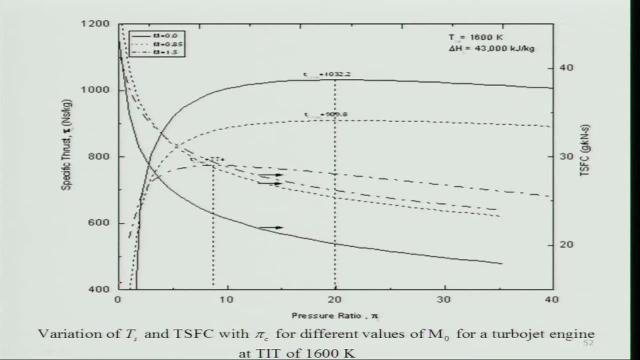 ratio across compressor. So 1 is the. you know that is. that means no compressor as such, right? So this value, it is going towards infinity, very, very large. it is having no meaning and you cannot have any meaning in turbojet engine having a pressure ratio of 1, right, ok, But 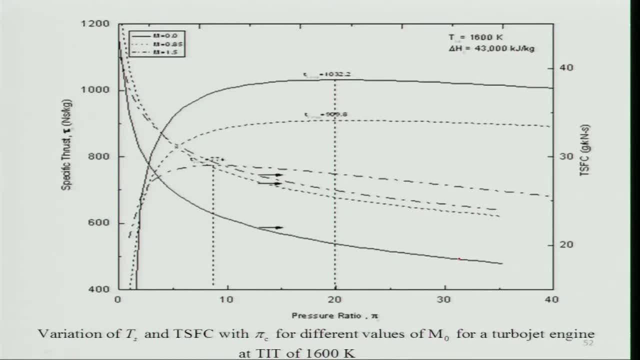 however, it decreases and you know it decreases continuously. as you increase in pressure ratio, you will see that this is having not a minimum values right. Unlike in a ramjet engine, there is a 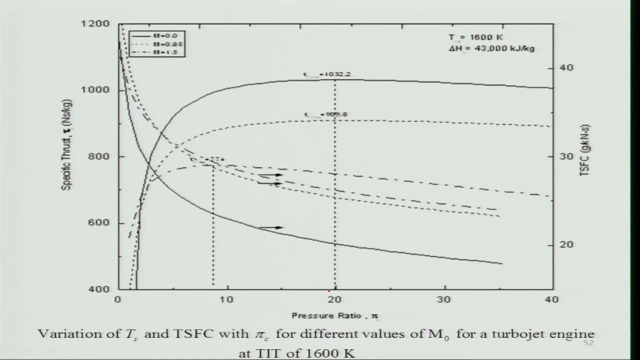 kind of thing where you get the maximum specific thrust, but if you go for a flight Mach number of 1.5, you will have similar features, right, similar nature of the curve, but only thing: it is decreasing. you know, after reaching a value of certain maximum value at a pressure. 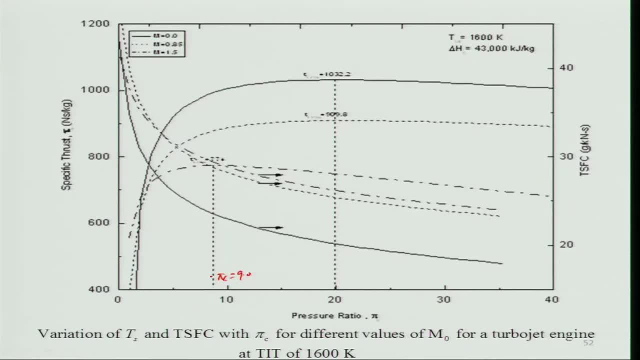 ratio of 9. phi c is equal to 9, you are having right. And then it decreases little, at a higher rate as compared to the more the sea level condition and or the static condition and the flight Mach number point. what it indicates. It indicates: 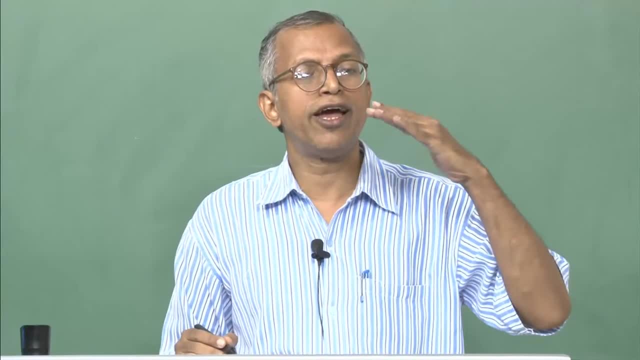 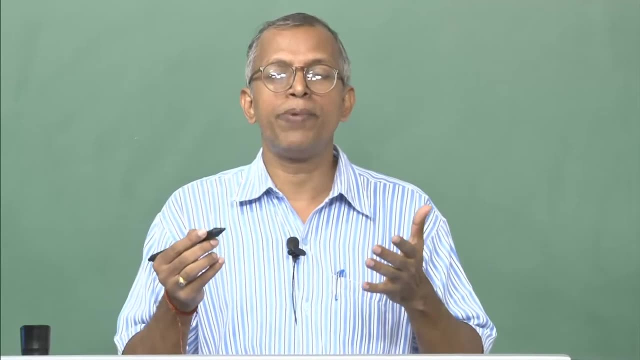 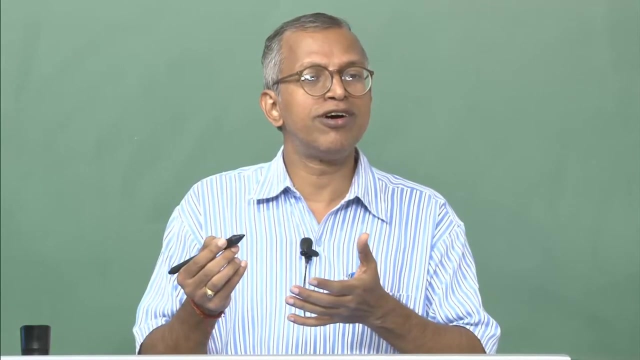 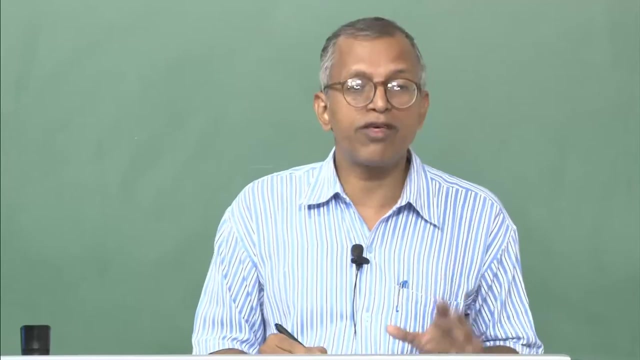 that when the flight or the engine is moving at a higher speed, it can use that pressure and you need Not to go for a, you know, high pressure ratio compression, because the ram pressure can be utilized right to, kind of, for increasing expression, right. So therefore it is, if you look at: 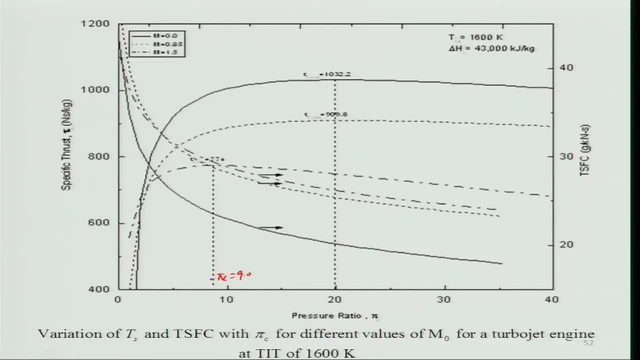 the fighter aircraft will be having a smaller compression because you need a very low pressure ratio, whereas you go for a long range passenger aircraft, you need to have a go for 20 kind of, But at the same time you will have to look at what specific thrust you need, because right, 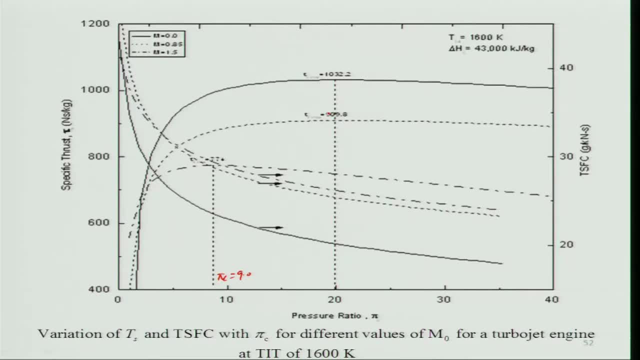 at a static condition with a static thrust is also important. So you will have to play around and see that what really you need and what is the level flight. So these are the things you can get by just doing. you know specific parametric analysis. right, that is. 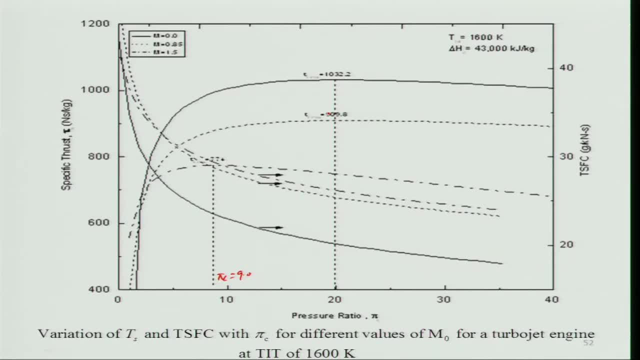 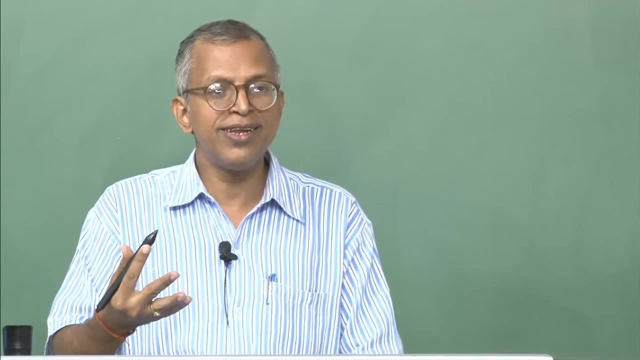 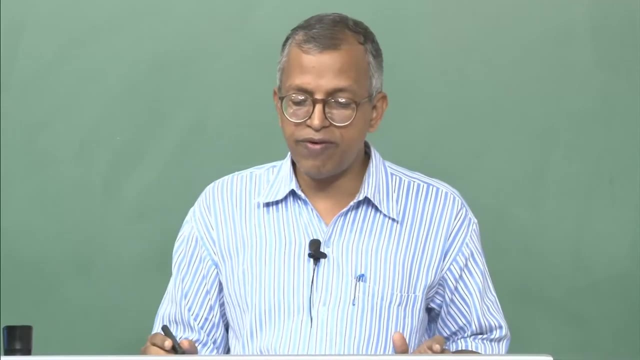 the beauty of this method that you can learn a lot by just playing around And see what is happening, why it is happening and what are the reason, whether you can have any scope to improve it further or not. So let us look at propulsive efficiency and the 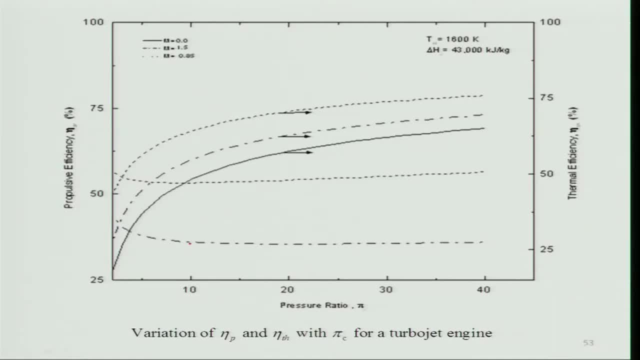 thermal efficiency. if you look at, these are the curves, which is, you know, basically the propulsive efficiency is two curves and it is a static condition. there will be no meaning of having propulsive efficiency when Mach number, type number, is equal to 0. So you, 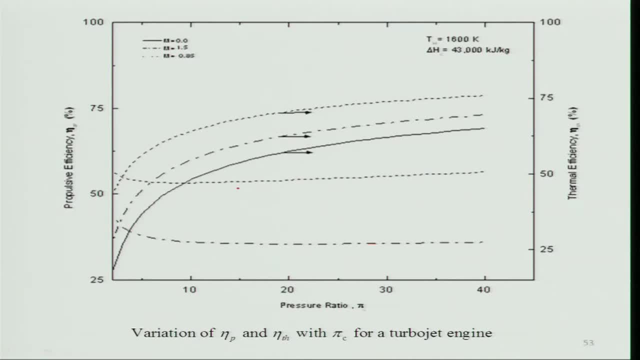 can take this and plot this as 1.5.. So this is a static condition, and it is a static condition and this is a static condition. So, whereas the what you call this one is basically Mach number of 0.85, it is having higher proper sin efficiency as compared to 1.5, right, but 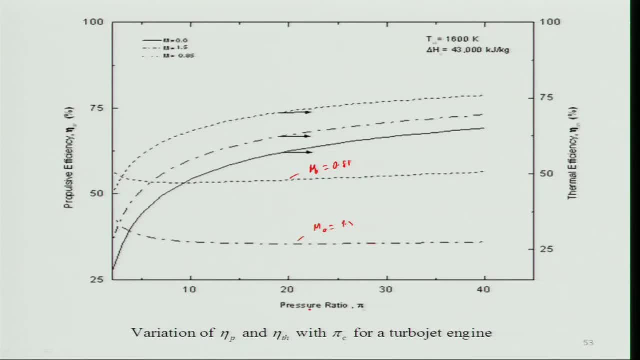 it is having similar features in the. when pressure ratio increases. right, it is very higher over here and decreases may be at certain pressure. it will just decrease. So you can minimum, which is not very obvious in this diagram, but when you look at number you get. 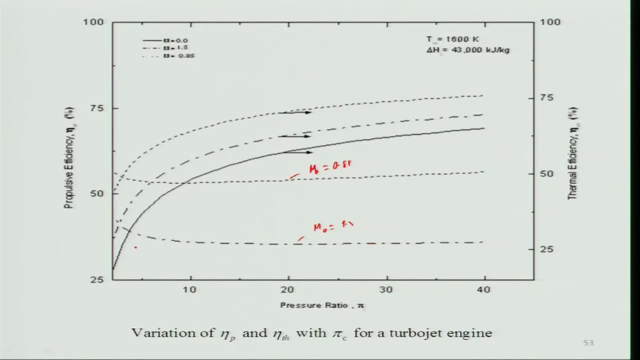 And thermal efficiency. it is goes on increasing, you know like, from the lower pressure ratio to higher pressure ratio and you will get a lower thermal efficiency. in case of, you know, 0 flight Mach number, and when you increases this 0.85, you know you will get a thermal